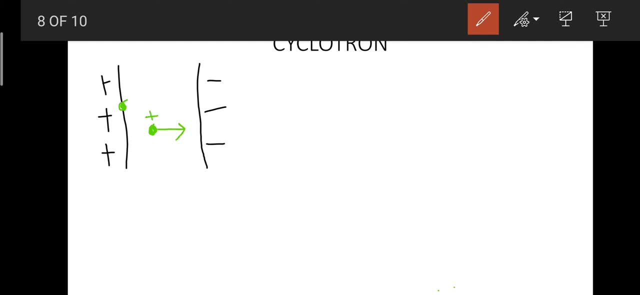 particle will definitely move towards the negative plate, away from the positive plate, right. So this is the velocity of this particular charge particle having charge Q. So in this condition, the force which is experienced by this charge particle would be equal to F, equals to QE, That is the electrostatic force, And because of this force it is accelerating in the forward direction. So, according to Newton's law, acceleration would be equal to F divided by. 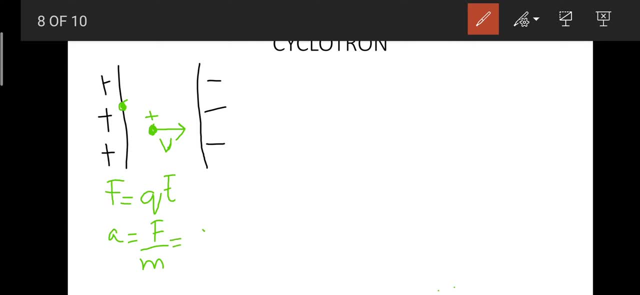 M right And putting the value of this F, what we are going to get we are getting QE divided by M. Now this acceleration is basically equal to QE divided by M and the velocity of this electron. acceleration of this electron. right Now we know that the velocity of this was the final velocity. initially, definitely, This charge particle was at rest, So the final velocity of this particle was originally soft. If you just take this off, move the particle down, And if this is not soft enough, if this is not still soft enough, that means that it will move자가. 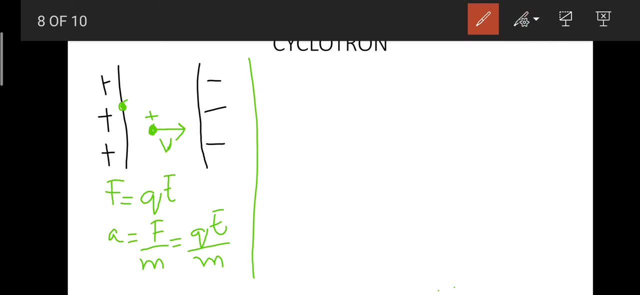 velocity of this was the final velocity initially. definitely, this charge particle was at rest, so the final velocity, which is equal to v, is going to be the velocity. so i'm going to write it like this, using the second equation of motion, which is going to be v: f equals to v, i plus 80 right. 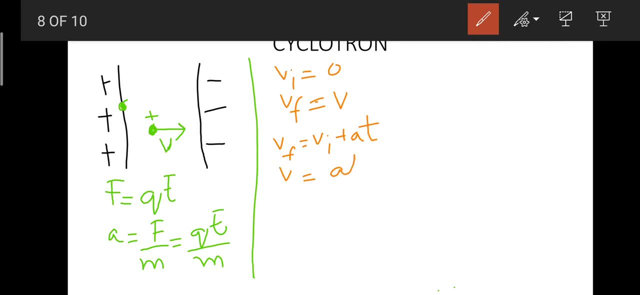 so v is equal to 80, since v i equals to 0. in this condition, if i'm going to put the value of a, this value, so v is equal to q e divided by m, multiplied by t. so that's how velocity can be calculated. i'm naming this equation as equation a right. 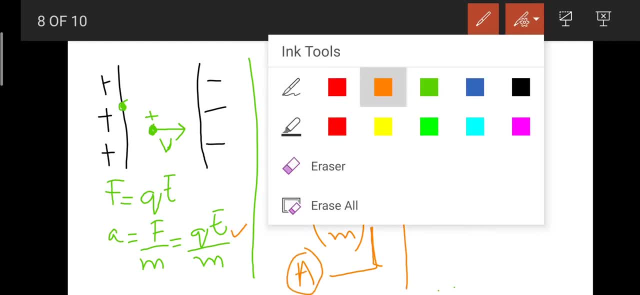 now moving towards the next step, since cyclotron is a device used to get the greater velocity of electron. so if I want to increase the velocity of the electron, what I need to do, I need to increase this T right, definitely, Q and M are constant. this is. 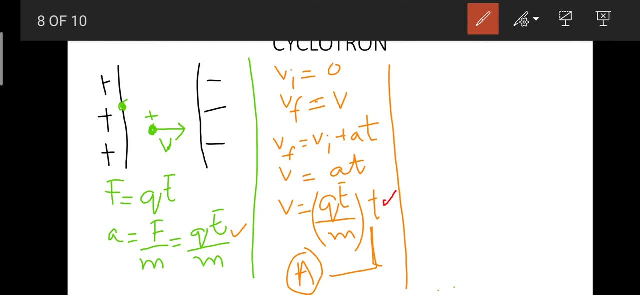 the specific charge and we are having E, it would definitely be constant. so if I want to calculate, keeping E constant, if I want to change, get the high velocity, I want a greater time period, so what would I do? I would definitely increase the distance between the charge plates. right, this is the positive charge plate. 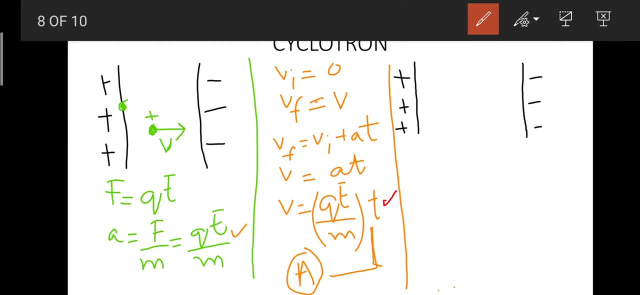 this is the negative charge plate and if I'm increasing this distance between them, which was initially less definitely, you can see from this state what is going to happen. like if I'm assigning the name as d1 and this is now d2, right, so we can clearly see that d2 is greater than d1. so in 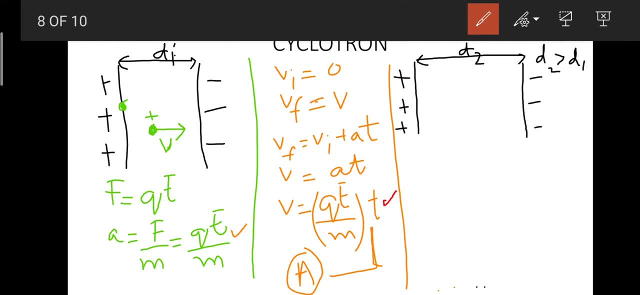 this situation, what is going to happen? that the time period will be greater, right, so the greater time period will be observed. so if initially the value of T were here was t1, so here at the time, or it would definitely be t2. likewise, if the time here is d2, I can see that the value of t1 is greater than d1, so here the time would definitely be t2. likewise, if the time here is d2, I. 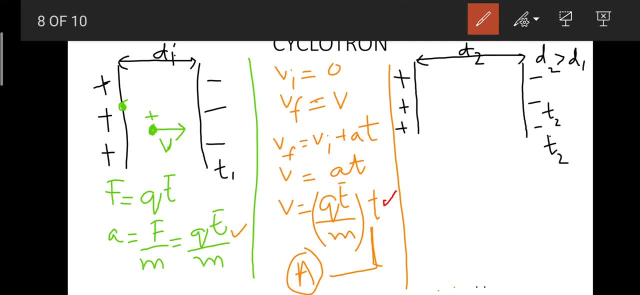 can write the situation. I can write: t2 is greater than t1. right to get this condition. I notice that if I'm increasing the value of T, the value of E decreases. why? because E depends upon the distance between the plates, directly. if I'm increasing, sorry, indirectly, so if I'm increasing the value of distance, 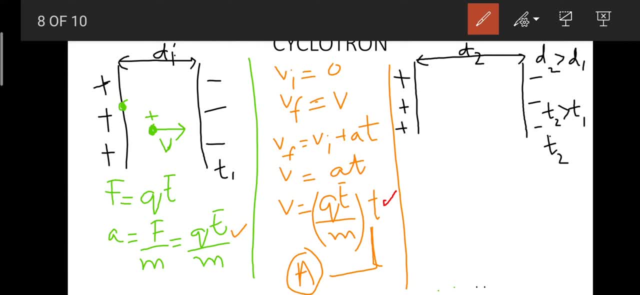 between the plates. what is going to happen? evil decrease, T would definitely increase, but in this case E would decrease. now, E if? now, if E decreases, we are not going to get the velocity to be greater. so we should increase E, right, since by the relation, by the formula of a potential gradient, E equals to V. 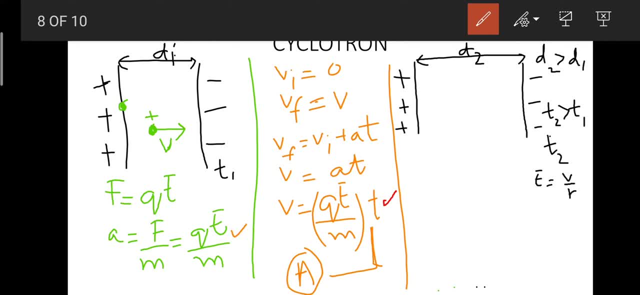 divided by R. from this relationship we can conclude that the value of V equals to E D. basically, V equals to E D. so this. so here B is the potential and R is the distance between distance and E is the electric field intensity. so they are having an inverse relationship. so, according to the formula which I am, 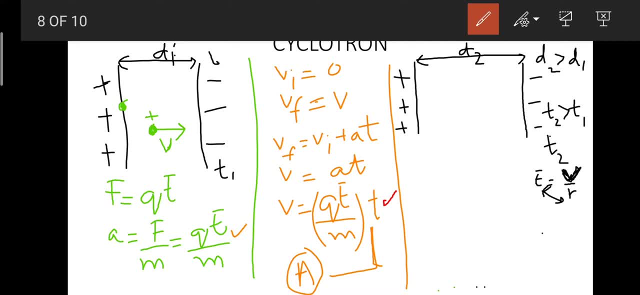 going to write at this point: e1 is equal to v divided by d1. and in this condition, what is going to happen? i can write: e2 equals to v divided by d2. so we see that if you are increasing the value of d in this figure, e2 would definitely decrease, right? so we can say that e2 is smaller than. 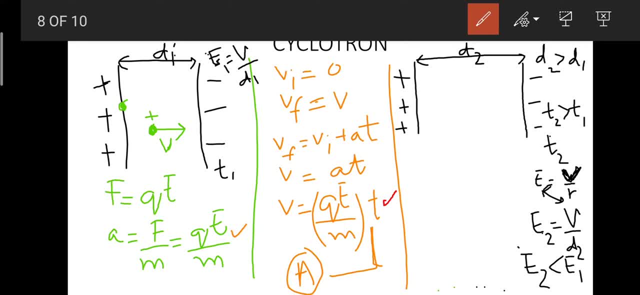 e1 right. so this is the main thing which is observed. if i'm going to increase, if i'm going to get a greater time, if i'm accelerating that charge particle for a greater time, so to increase e, what i'm going to do to increase e, i'm going to do this thing that i'm going to. 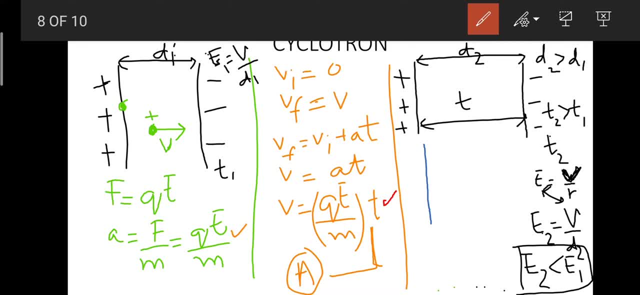 decrease this particular distance between the charge particles. now we can see that i have decreased the value. now, if i've decreased the value- that is, the decrease, the distance between the charge plates- what is going to happen? i have decreased e. that means e has increased. so in this condition i can write. e will definitely. 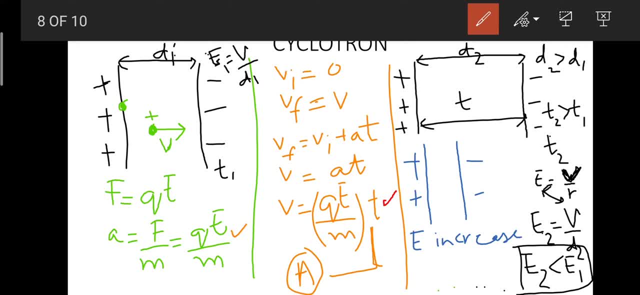 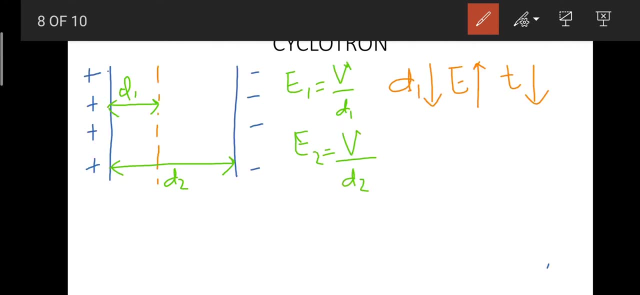 increase in this situation, but time experienced by that charge, particle would decrease, right? so in this condition, again, velocity cannot be increased, right? so what we are going to do? so i've drawn a figure, a clear, much clearer figure, and combined figure as well. so there is a distance- d1, which is the smaller one, and there is a distance. 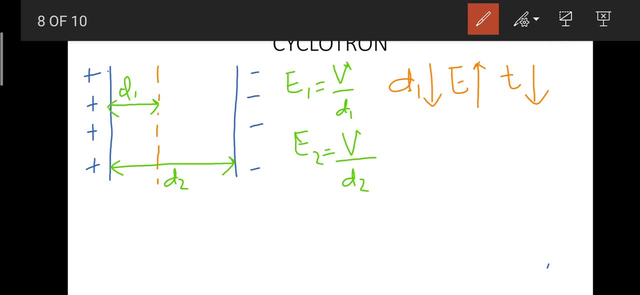 d2, which is the greater distance. i'm going to do explain for both of them. if d1 is like d1 is smaller, if i've put the charge plate close to the other plate, if i've decreased this distance, i've put the negative charge plate at this particular point, what is going to happen? 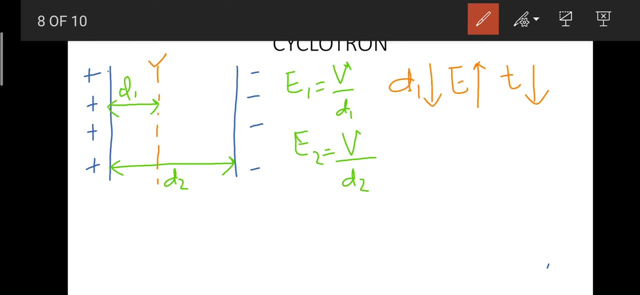 d1 will definitely is less. if the value of d1 is less, then according to this uh inverse relationship e1 is definitely going to increase and because of the relation x equals to vt, what is going to happen? the value of t will also decrease. in the second situation, what is going to happen if i'm 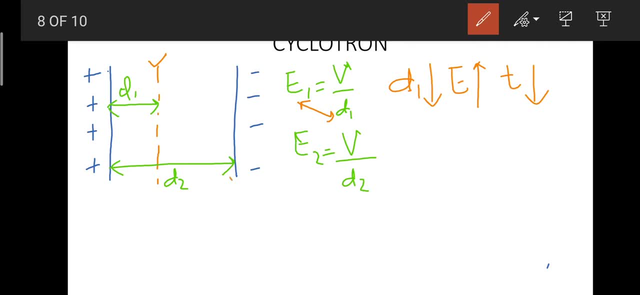 if i'm going to put this plate at this particular point. negative plate has been replaced at a far distance. uh, the now the new distance is d2, if the value of d2 is greater now. so, according to this relation, if d2 is greater that means t is greater, there is more time achieved, but the value 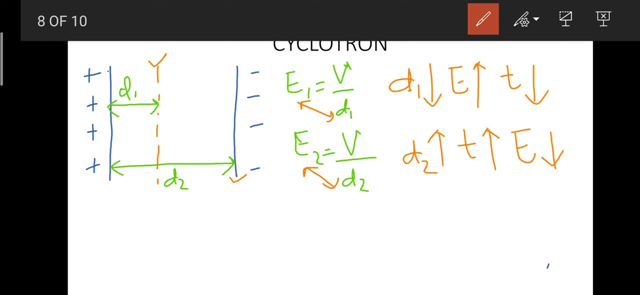 of e has been decreased. so in this situation, we are not going to get v to be very greater, right, but i need to achieve velocity to be greater. so to um, what should we do in this situation? um, we are going to do one simple thing. i will draw the diagram so, as you can see in this figure, if i'm having a charge, particle. 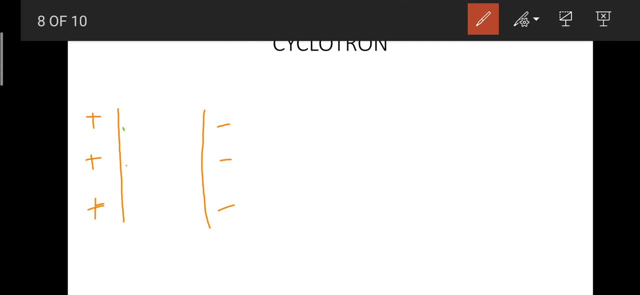 like, at this point, a positive charge particle. then what is going to happen? this charge particle will definitely move towards the negative plate, and when it moves towards the negative plate, what is going to happen? so consider: initially the velocity of this charge particle was zero and after it is moving towards the negative plate, definitely its velocity is. 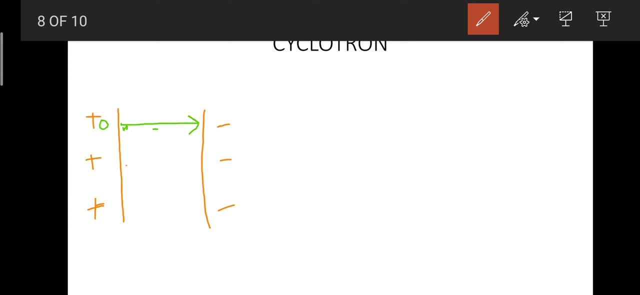 increasing and consider that after reaching this particular negative plate its value of velocity gets v. now consider there is another charge particle. if it is moving the velocity v and if it accelerates in this particular electric field, after some time its velocity becomes 2v. and consider there is another charge particle whose velocity 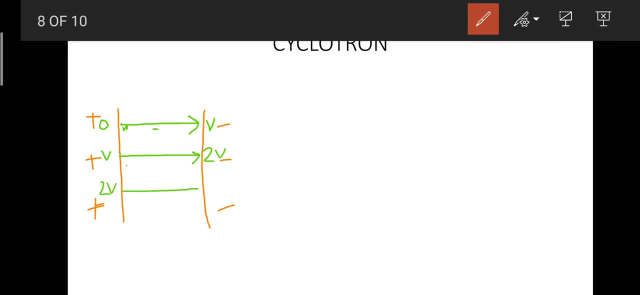 was initially 2v, so after accelerating in this electric field, its velocity is going to be increased. and consider this velocity to be 3v now. consider that this particular, in this particular field, there are some more charges, more and more, more charges. again and again, charges are moving. 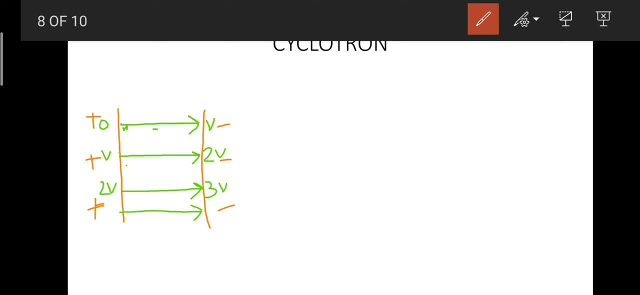 so, uh, consider that the final velocity we achieve for the electron is going to be thousand v, equal to thousand v. then imagine what sort of kinetic energy we are going to get for this, uh, thousand, uh, world, thousand times velocity of that particle. so the final velocity we achieve for this particle is going to be a very big value, right? so, um, if i 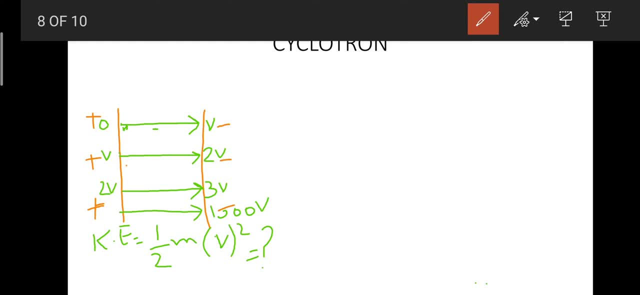 really want to get a high energy or high velocity particles. what i am going to do, we will definitely going to do this thing that, as this charge particle is moving forward in this particular direction, if i in any means, by any means, if i um to introduce this charged particle on this particular point, like at this particular point, 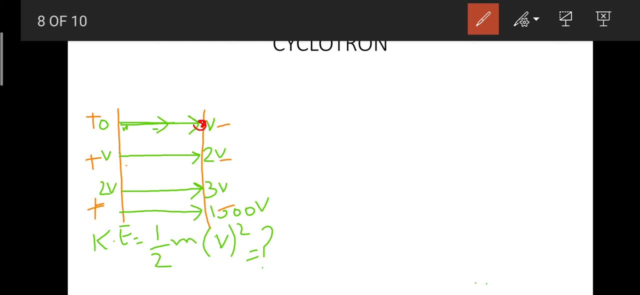 if i really can enter the charged particle back into the field, like again back into this particular field. so then its velocity was initially v and then, by increasing its velocity as it is getting higher and higher, it is getting 2v velocity. now, if i use the same 2v velocity electron or the 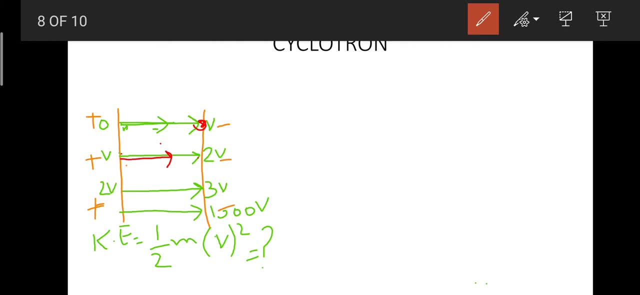 charged particle or any particle. what is going to happen if it is again introduced in the same electric field? its velocity would become three volts. now if again i introduce this three volt, three times of velocity of the, the charged particles, again into this electric field, what is going to happen? the velocity would 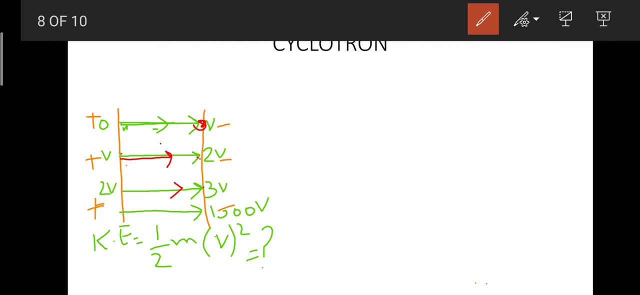 increase to the four v. if i again introduce this particular charge particle in this field, what is going to happen? its velocity would increase and we get 5v. then 5v would become 6v if again introduced. so basically what we want we are. we actually want to bring this charged particle. 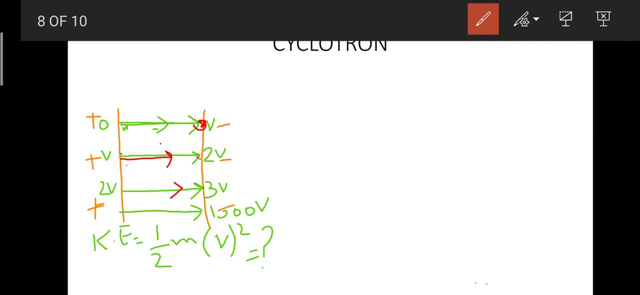 again and again into this electric field. what is going to happen if i am introducing this charged particle again and again electric field? its velocity is increasing, as you can see from this figure right. so how can we bring the charged particle again and again into this electric field? so to get this particular stuff now we require the magnetic field. basically magnetic force would result in moving that charge particle again and again into this electric field. so to get this particular stuff now we require the magnetic field. basically magnetic force would result in moving that charge particle again and again into this electric field. so to get this particular stuff now we require the magnetic field. basically magnetic force would result in moving that charge particle again and again into this electric field. so to get this particular stuff now we require the magnetic field. basically magnetic force would result in moving that charge particle again and again into this electric field. so to get this particular stuff now we require the magnetic field. basically magnetic force would result in moving that charge particle again and again into this electric field. so to get this particular stuff now we require the magnetic field. basically magnetic force would result in moving that charge particle again and again into this electric field. so to get this particular 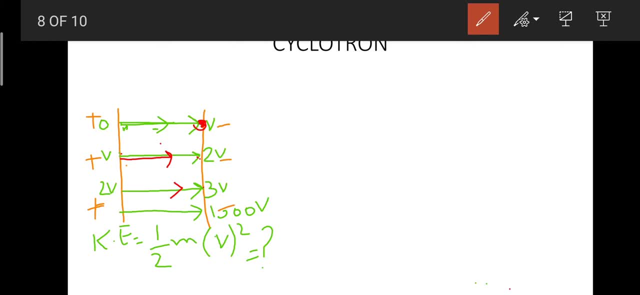 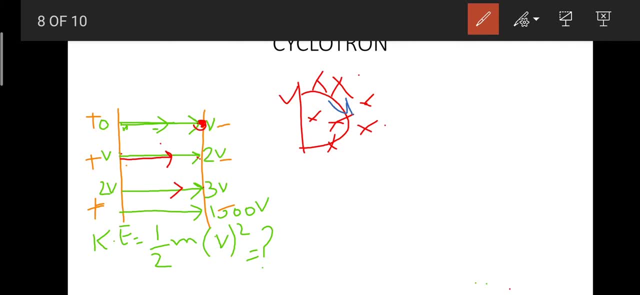 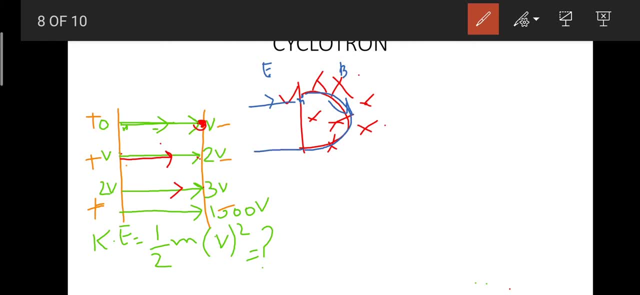 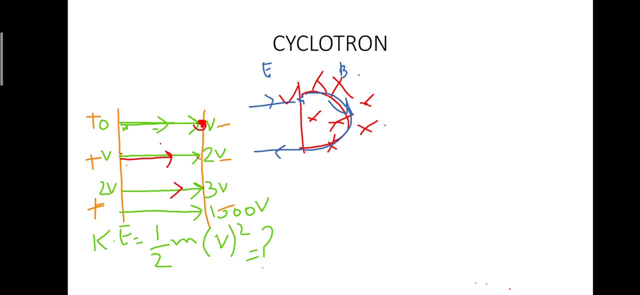 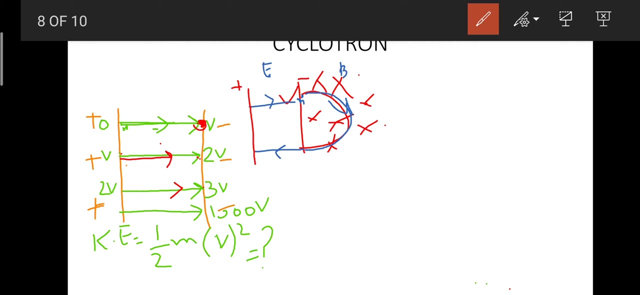 uh, enter in this particular electric field right in this way and again, uh, there was. so we can see. the charged particle is moving towards the next plate, that is, the positive one. and in this positive plate, what is going to happen? i'm again going to provide magnetic field in this region. so what is going to happen? that the path of this particular 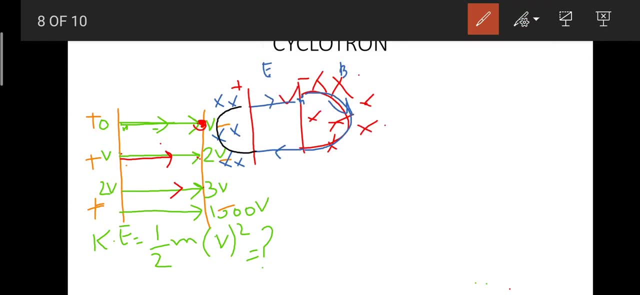 charged particle is again going to be the curved one. so basically what we are doing, we are introducing this charged particle again and again into this electric field. electric field is basically going to increase the velocity of this charge, that charge particle, and b, that is the magnetic force, is responsible to move that charge particle. 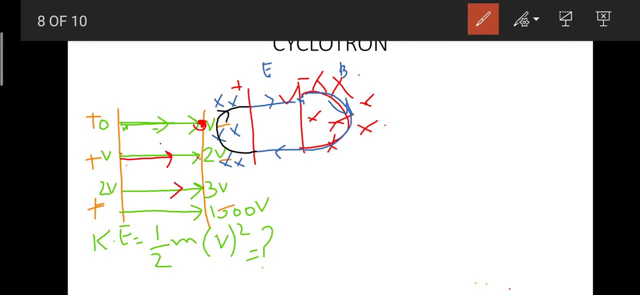 back into the electric field because it curves the path of the charged particle. so that's how we are again and again going to get the charged particle back into the electric field to increase its velocity, right? so this is the principle on which this cyclotron works, in which e basically elect. 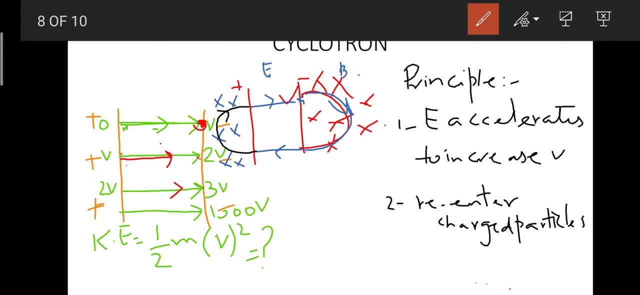 accelerates the charge particle particles to increase v, um and the magnetic field. what it is doing? it will re-enter the charged particles into the electric field. so both electric and magnetic field um is going to work over in this particular device which is known as the cyclotron, now um, and the device itself. 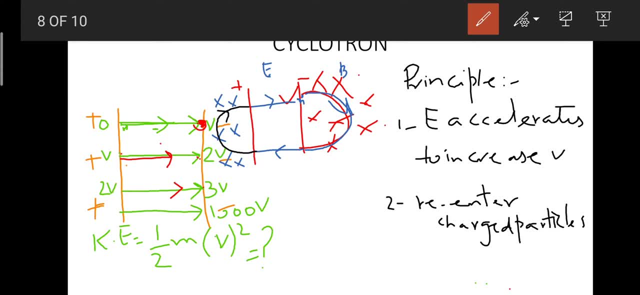 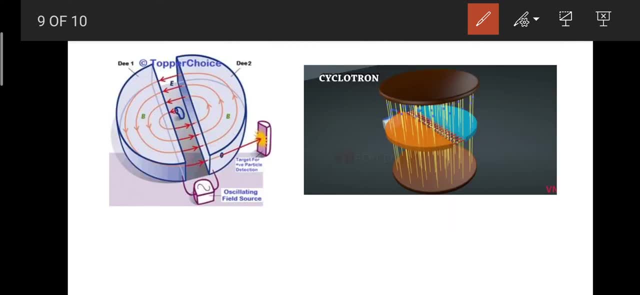 how we can draw it. so, to draw that device, i am going to see. so this is basically the actual figure of cyclotron, right? not an actual figure? this is basically a visual representation of cyclotron in which you can see that there are basically uh, two uh, d's. like. what is d uh? if you are having a circular path, like a circle, like uh, consider, 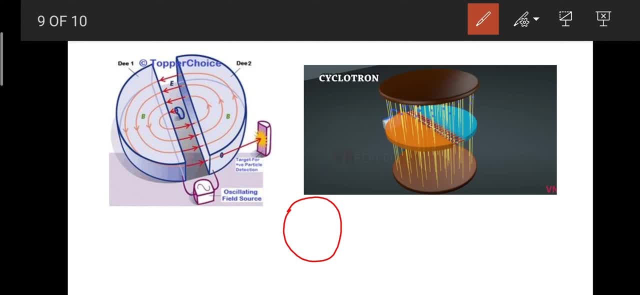 there is a disc you are having. if you divide that disc into two equal parts parts, right, what is going to happen? we are going to get two d's like this: okay, so this is d1 and this is d2. uh, so we are having now two d's, uh, as indicated, as you can see, uh here in the orange. 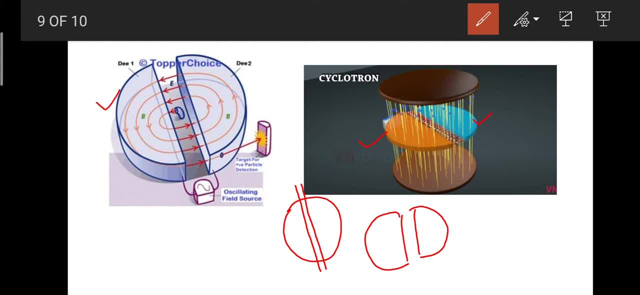 color and here, in the blue color, or in this figure again, we are having d1 and here it is d2. so in this, uh, in this figure, you can see that between these, uh, these, we are having an electric field. like, suppose, uh, we are having an electric field, um, in any direction, like, if i consider this direction, the field is going to be. 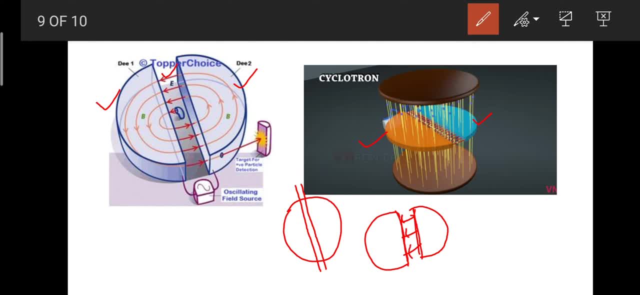 from this point to this point. likewise, that means we are having a positive plate is right here and a negative plate is in this, in, on this side, right, um, so like, direction of electric field is towards the left side, um, as you can see that there is a little thing which is placed in this central point, this, what? 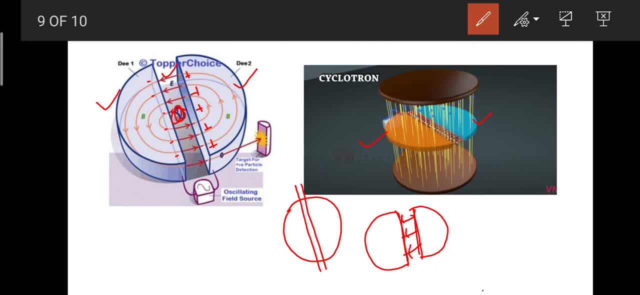 is this? this is basically an ion source right in the center of these two d's. we basically place the these two d's directly on the top. now, what great yourself that you know. yeah, i don't know, i didn't even realize that. right, and even though it was not an ionage, so it was a very similar uh. 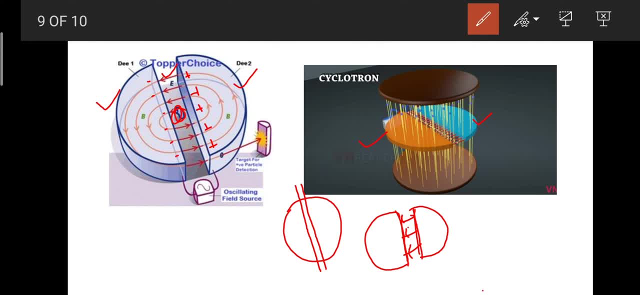 organizating the uh iris from the ground up. just lifting up, looking at the food and giving you better idea also of you. have this number right. what is dizzy either? what is the ion source of the earth and overall, here we are having that too. okay, in that, uh j uplift, it is a. 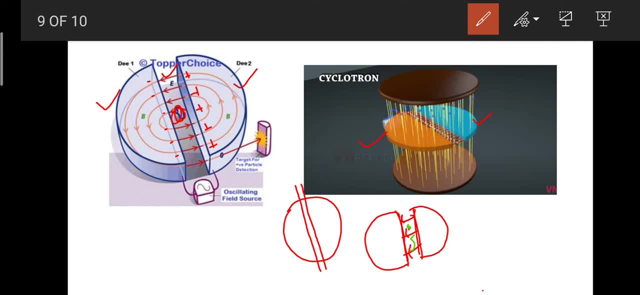 energy source. this is essentially the temperature value. this is going to say the type of uh this Store right at this moment. section f is calculate that. so it is a normal temperature. that is the source. okay, so the not attorneys suppose that means that this f is supposed to be 28 degrees, so that your heat making things. 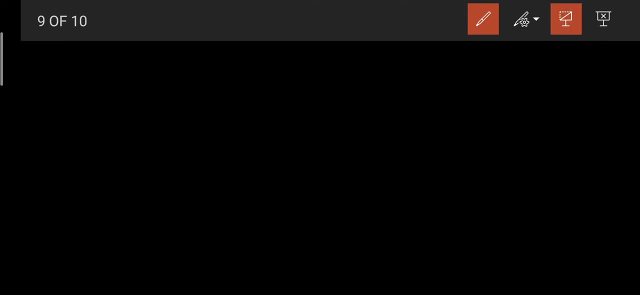 Now coming towards the fact. So I have drawn another figure. In this figure you can see that we are having the 2Ds and a magnetic field has been supplied to it, and these 2Ds are connected to an external source. This source must be an alternating source, So this is known as alternating source oscillator, or you can simply call it oscillator. And since this is an alternating source, so what is going to happen Then? the polarity will definitely be changed after the every half cycle. 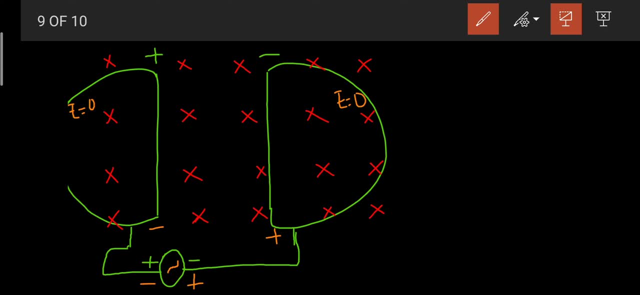 So what use is going to be we are having because of this oscillator? I am going to explain it later. But firstly, consider the fact that this oscillator is going to have a very, very high voltage. that is approximately 10 raise to power, 4 volts, and the frequency it is going to have is definitely going to be definitely very high. That is 10 raise to power, 6 hertz. right, What does this mean? I will explain that later, after you perform this whole experiment. 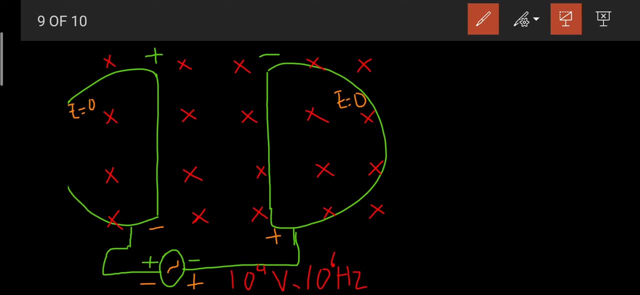 So, in this configuration, what is going to happen? For the first half, we are going to have this particular plate to be positive, right, And the other plate would be negative. But for the second half, what is going to happen? this: this plate would become negative and the other plate would become positive. So this polarity will change according to the situation. 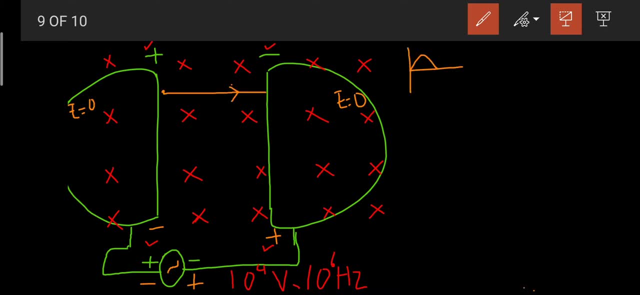 Okay, So consider that we are having A positive, positive charge particle right at this point, and this charge particle will move away from the positive plate and move towards the negative plate. during this movement, its velocity is going to be increased. right now. what is going to happen? uh, the velocity of this particular 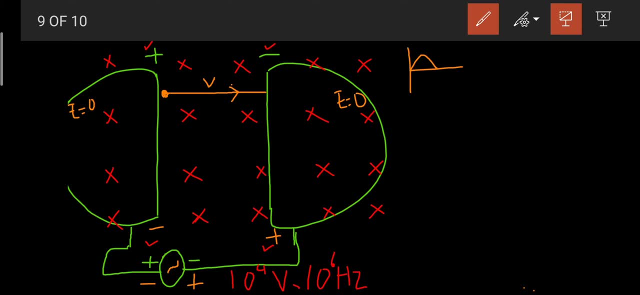 like, wait, i need to draw it a little bit lower. yes, so i have drawn it a little um lower. what is going to happen? that from zero velocity, that charge particle, which is positively charged particle, it will move in the forward direction under the influence of electric field. 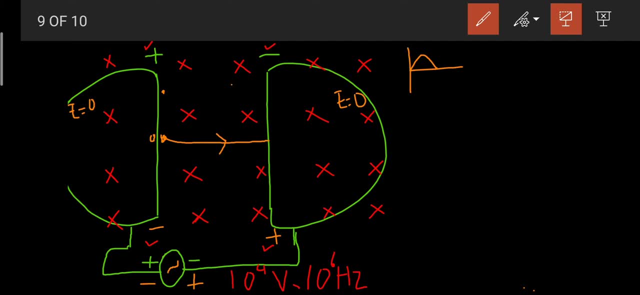 and reach to the other point of the d? um, towards the negative plate. now what is going to happen is that the charge particle will move away from the positive plate and going to happen over here that its velocity has increased. and consider that velocity is now, uh to. 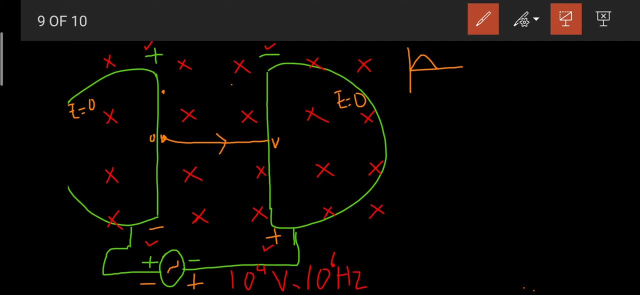 be v? now it will definitely. this electron will definitely enter into the um d. this, when this charge particles, uh, enters the d, what is going to happen? it will experience the um magnetic force and, okay, so it will experience a magnetic force and it's a linear path- will be. 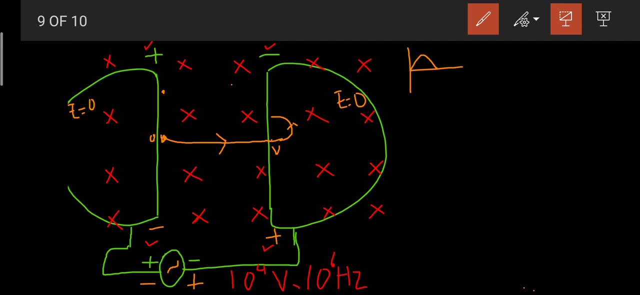 now be curved and it will again enter into the electric field. right now, as it moves in this electric field, its path would be like this: it will move forward in this particular point right, and this is going to be happen. uh, you must be wondering that, why it is not. 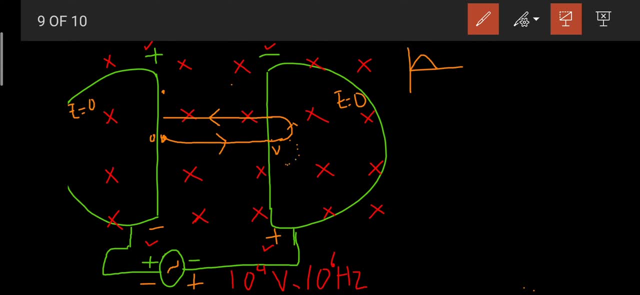 moving in this particular direction, that we can draw it in this direction. why it is not going to happen, it's because of the fleming's left hand rule, because magnetic force, how it is experiences, since the direction of b is towards the negative z and the direction of velocity is in the x-axis. 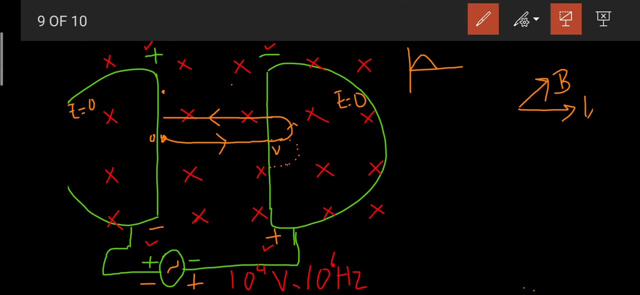 direction. so the direction of uh force, that is, the magnetic force, would be in the like. it would be in the upward direction. so that's why this particular charge particle- positively charged particle- will have a motion in the upward direction and again its path will be curved um, and that's how it will again enter into the magnetic field with velocity v right. 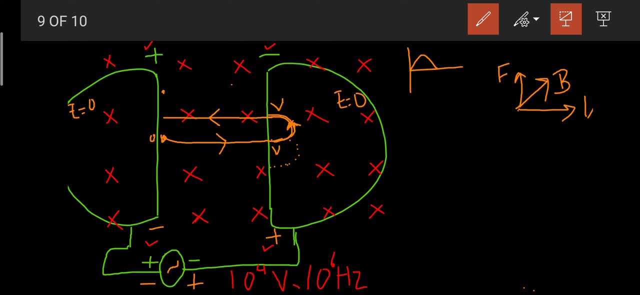 in the d there is no electric field, so its velocity would won't be increased. uh, as it will move in the forward direction, it will experience the electrostatic force. because of that its velocity is increased, and when it reached the other part of the d, its velocity- consider its velocity- has. 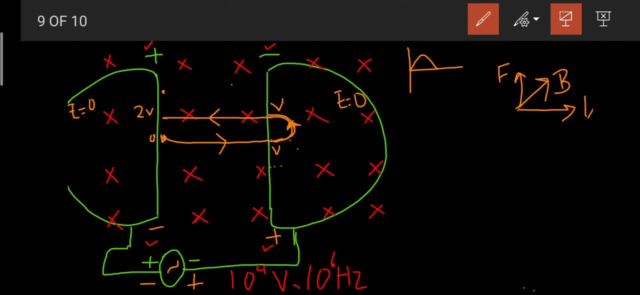 now become 2 v. okay, so at 2 v um, what is going to happen? that a charged particle would again entering into the d. so there will be no electric field, only a magnetic field is there. so the path uh, charge um, charge particle uh would now be greater. why? because now the velocity is greater. 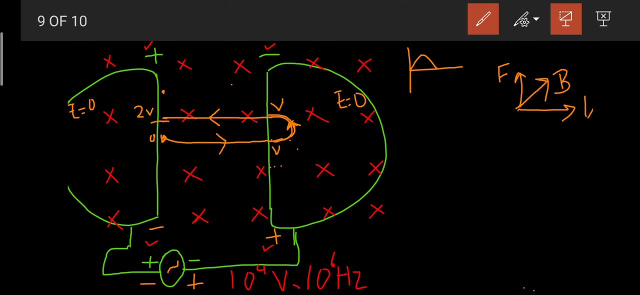 so definitely, the radius would also be greater. so what is going to happen? it is going to have a greater radius this time and it will again ready to enter at the velocity of 2v back into the electric field. so when it enters again into this electric field, its velocity will increase. 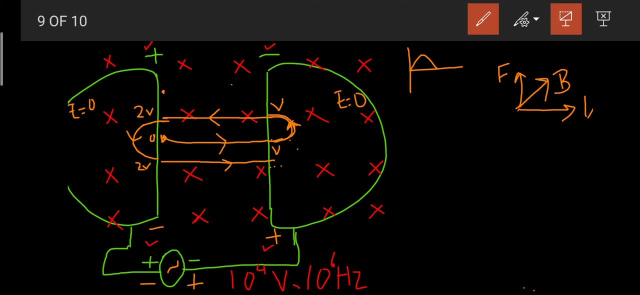 and it reaches the other part of the uh d at a velocity of- consider 3v right. and again, what is going to happen? since its velocity has increased, so its radius will also increase. so with the greater radius it enters this particular um electric field, again with a velocity of 3v. so again, when it enters this electric field, its 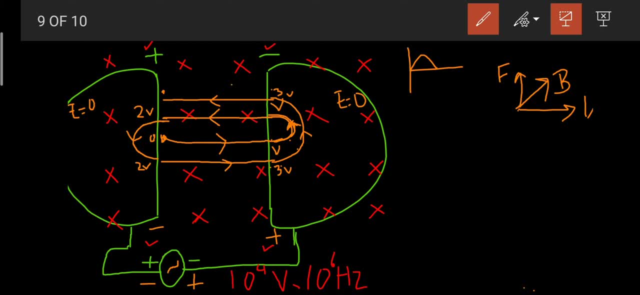 velocity is going to increase again um. and it will read: suppose at this particular point, with a velocity of, suppose the value of this velocity is 4v um. and again, because it is having a greater velocity, so its radius is now also greater, it enters the field at electric field, at this particular velocity of 4v. again it enters the 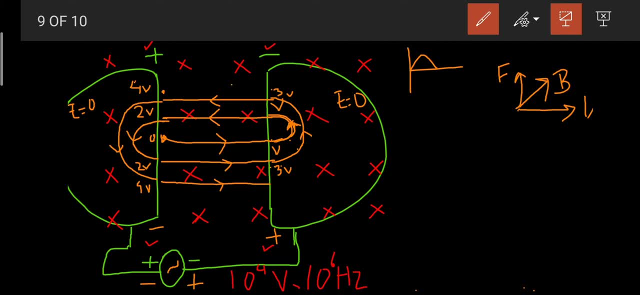 electric field, its velocity is again increasing. um so consider, at this particular point, its velocity is 5 volts. so it again enters into the achieving a higher radius because of greater velocity. uh, again, at this point, its velocity is 5 volts, it's going to enter the 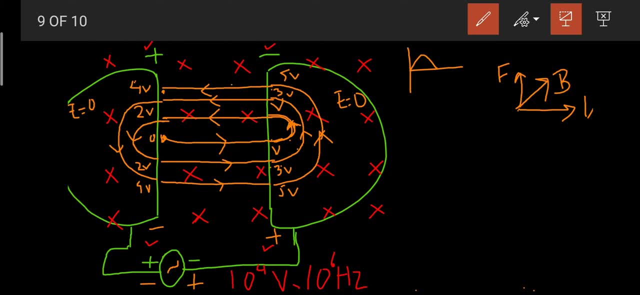 um electric field again and velocity would definitely increase. consider this velocity to be six volts. right, velocity, greater. definitely radius would also be greater. it again enters into the field at a velocity of 6 V and when it reaches to the other part of the D its velocity has been increased. consider it to be 7 V, and again, and again, and again. 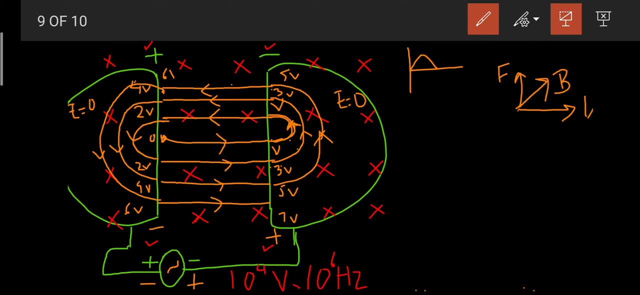 that's how we can increase the velocity of electrons up to thousands of thousand times of the initial velocity. so how this is going to be increased? because of the electric field. right, electric field increases the velocity and magnetic field is basically putting back this charged particle again into the electric 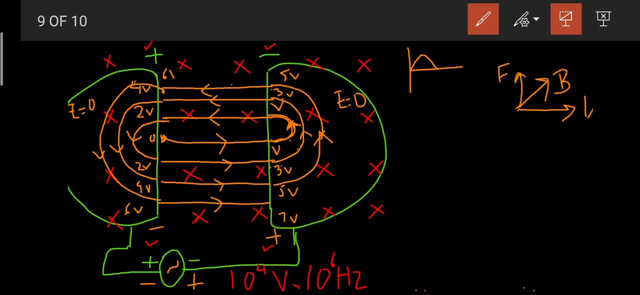 field. now consider that at the final point the velocity has been increased so much to our desired value. what is going to happen? so what is going? suppose I want the particle to be received at the velocity of 7 V. 7 V is also a very small value. I want to be. 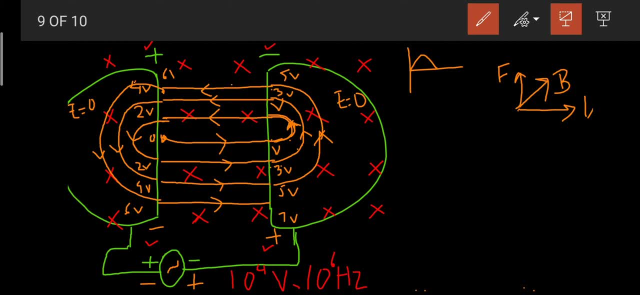 received it as, suppose, at the value of thousand V. so when I receive, how can I receive that particular charged particle? what is going to happen? that there would be a small window, this particular point, there is a window and through this window there is full target. right, there is a target at which these charge particles are going ahead. 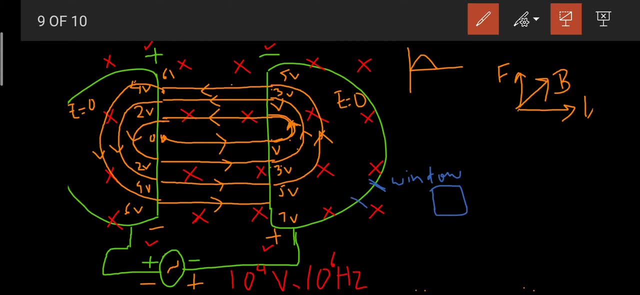 so these ions will definitely, they will move towards this particular source and they will definitely move out of that window and reach to this particular target. right, and that's how we can receive all the charged particles with a greater velocity in this way. now consider that all the electrons- sorry, all of the charged particles- are having a cyclotron motion, right? 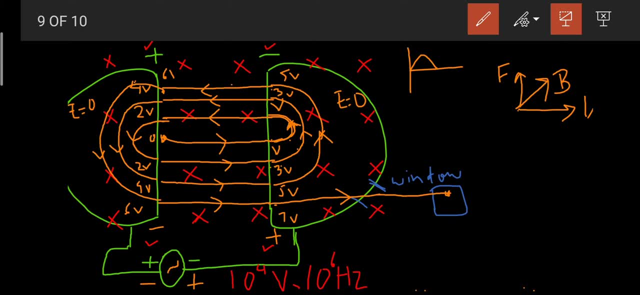 so you must be wondering what is the purpose of, um, having this, uh oscillator, that the polarity is going to be reversed, uh, what is the purpose of that? so, um, to get the purpose, i am going to uh describe it in this way, uh, to understand that thing thing, consider that. 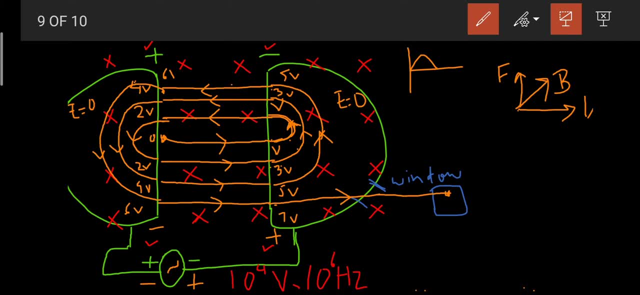 the charged particle is moving from the positive uh plate um to the negative one, right in this positive x-axis direction towards the right side. now, if it is moving from this point to that point and when it enters again into that particular field, now, in this condition, if the charge plates 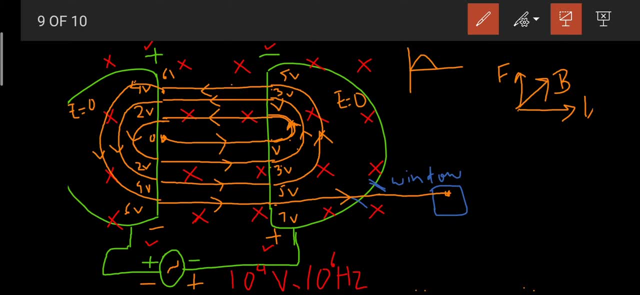 are in the same way, then that charge particle, which is basically the positive charge particle, it will be like, suppose, if it at this point, so this charge particle has to do this charge particle, it has to do work since it is having a positive charge. so, and this is, it is on the 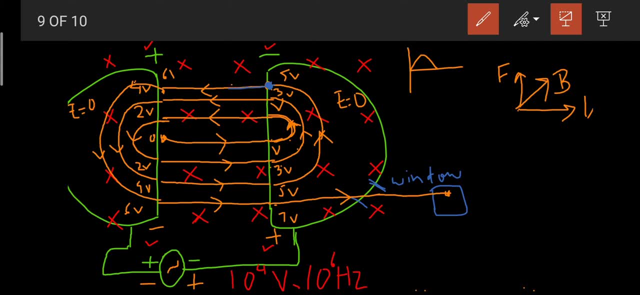 negative plate. so it has to do a lot of work to move uh opposite to the electric field, since the direction of electric field is in this here like towards the right side. so this charged particle, that is, the positively charged particle, has to do a lot of work to move away from the negative plate. 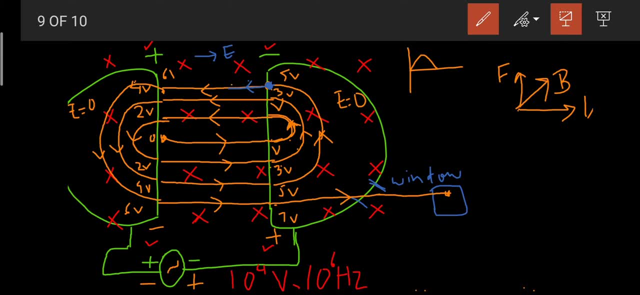 and moving towards the positive plate. so this will definitely reduce the velocity. now, if the velocity is getting reduced, then how we can get the velocity to be greater so every time the charged particle will turn back, its velocity would decrease in this case. why? because, if you are, if at this particular 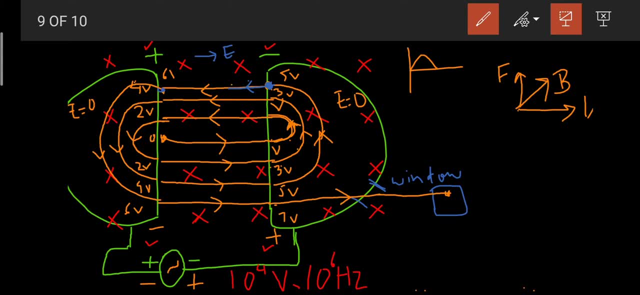 point right. if the charge particle reaches after getting a lower velocity, its velocity has been decreased and it reaches at this particular point. when it reaches this particular point, it will again enter into the magnetic electric field and, moving towards, like moving in this particular direction, its velocity would increase, reaching at this particular point. 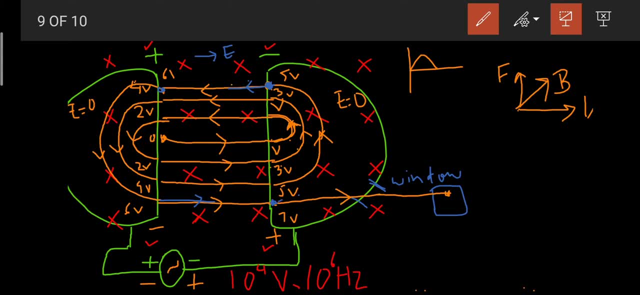 its velocity has been increased. but again, when it again enter into the circuit, its velocity is going to be decreased. right when it is, it definitely. when it reaches at this particular point, it's velocity is again going to decrease. so velocity is increasing and then it is decreasing, then 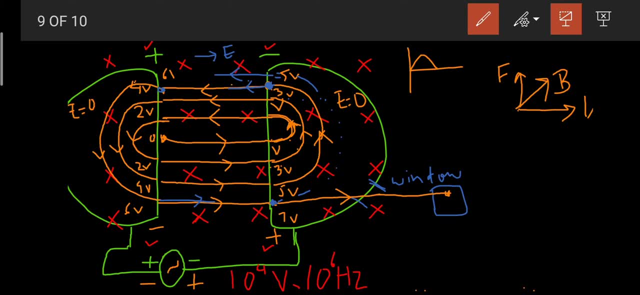 how we are going to get the increased velocity. so, uh, to avoid this we are, we have to synchronize v and e, right, and how this synchronization will occur. to understand that thing, uh, thing, you uh should keep this thing in mind that we have to calculate the time period for the charge particle. 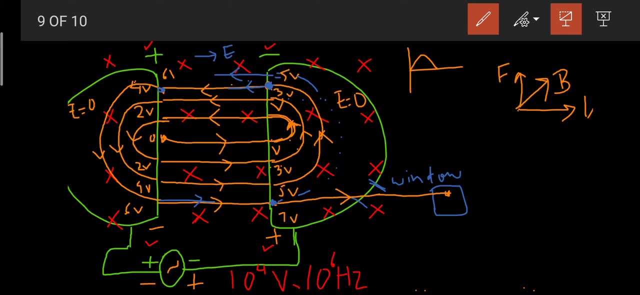 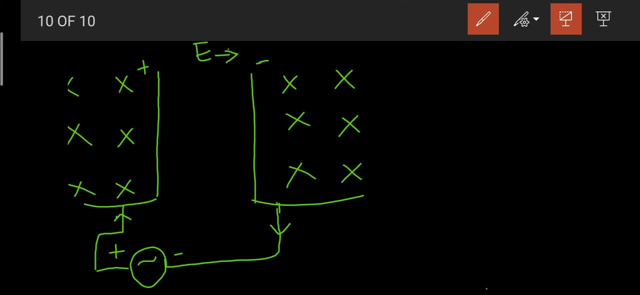 and then set the oscillator to change the polarity after that time period. so, in this case, what is going to happen? the charge particle will definitely move towards this side, right to get the synchronization effect. uh, we to get v and e to be synchronized. what we are going to do? um, we are going to calculate. 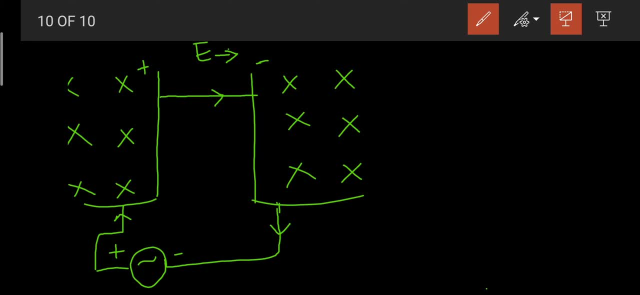 the value for the time period. uh, so to understand that thing, the charge particle will move into the electric field and after reaching the other side of the d, it will be having a curved path and it will again re-enter this particular electric field to avoid the decrease in velocity. 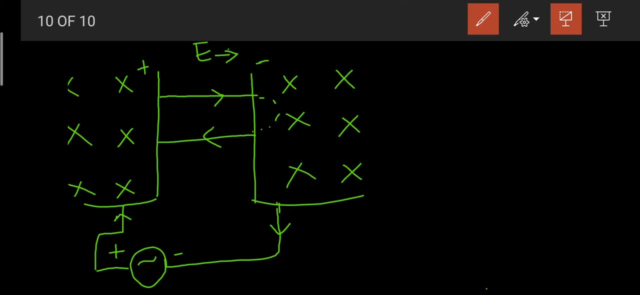 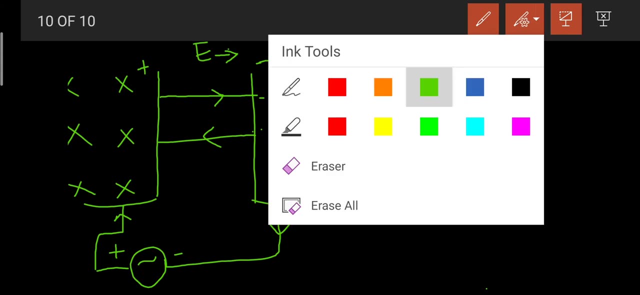 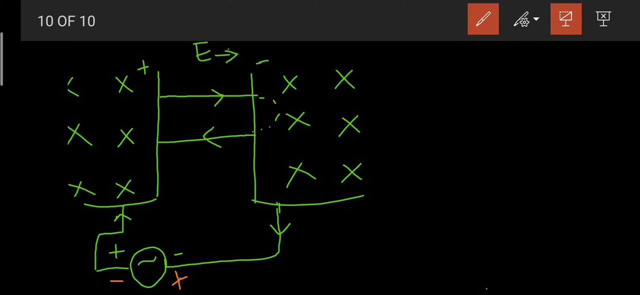 in this situation, what we do? we basically change the polarity of the oscillator. if the polarity of the oscillator is changed in this situation, what is going to happen? that now for the second case, when it is moving back into this electric field. when it is moving back into this electric field. 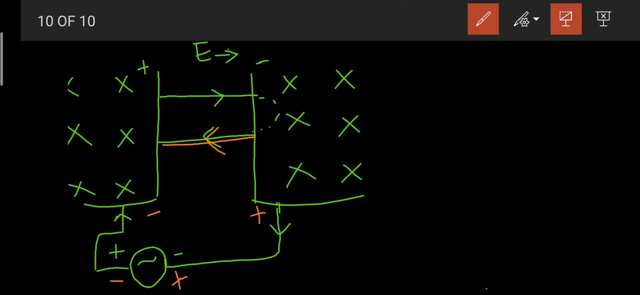 what is going to happen? this plate would become positive and this plate would become negative, right, uh, when this plate becomes positive, definitely the positive charge is there. so positive charge will move away from the plate and, uh, it will reach to the other side of the t. in this condition, it does not have to do any kind of work. so 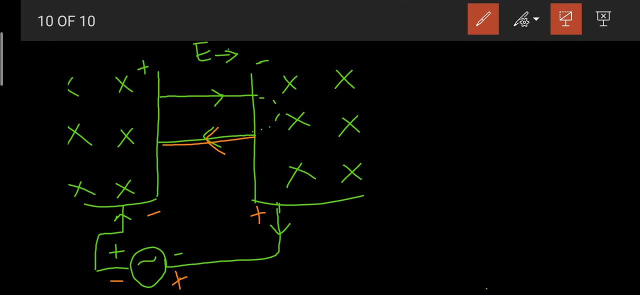 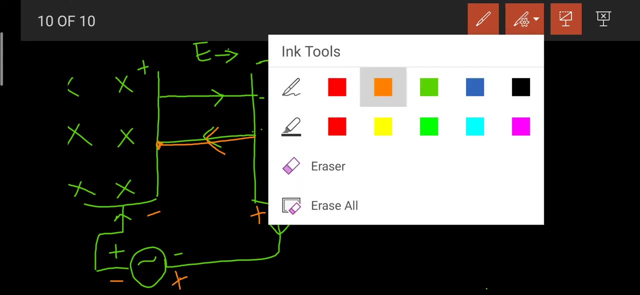 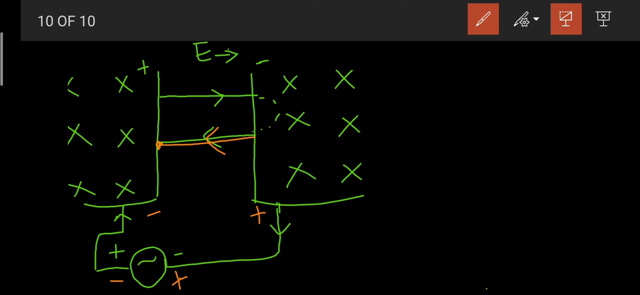 velocity would definitely increase right now. again, what is going to happen? at this particular point? the polarity would again reverse, and when the polarity reverses, this is going to be the positive plate. right, this plate would now be the positive plate and the other plate would be the considered. 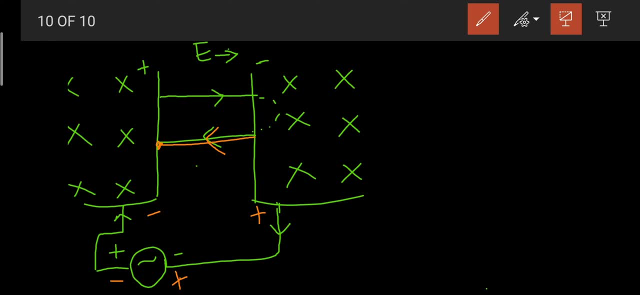 as negative plate. so the direction of charge particle would be like this: there would be no increase, sorry, there would be no requirement of doing the work done right again when it is going to enter this particular electric field. what is going to happen? this, this fact would be done by 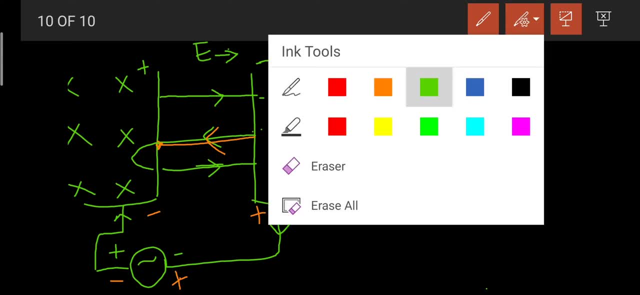 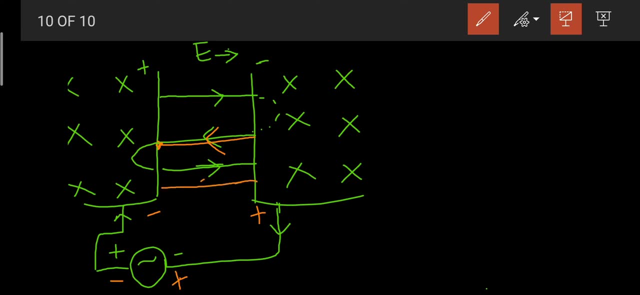 changing the polarities. and when the polarities are changed it will come back into this particular electric field in this condition. so all the lines which I have drawn, orange for this kind of case, what is going to happen? the polarity is would be the change one, and all the green lines show that the polarity is B is from, like electric field is from. 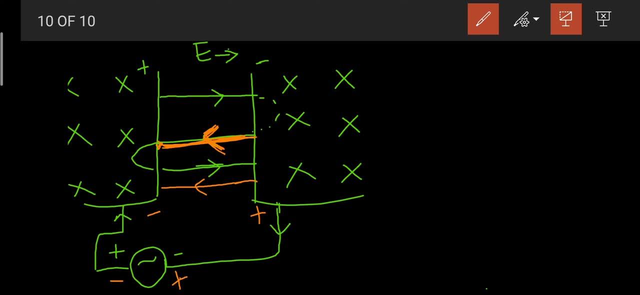 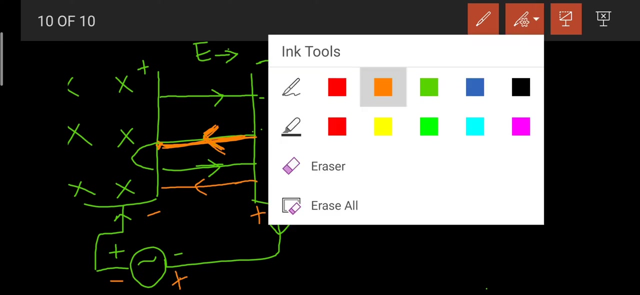 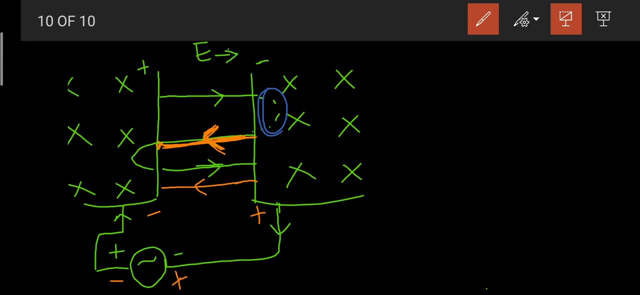 left to right right and for the orange lines case we are having that the polarity is from right to left. now this condition can be achieved, but we have to make sure that the time which which a charge particle is taken, taking at this region in the D, should be equal to the time when the polarity is going to reverse. 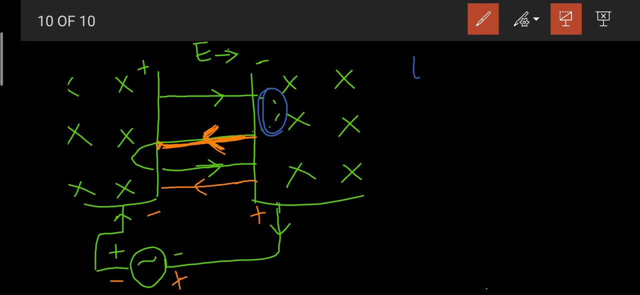 right. so the time taken by this time, which is taken by the charge particle in the d, to get a curve and then again get to enter in the magnet electric field, this time should be equal to the time which is taken by the battery to reverse its polarity. right, so t and t prime should be equal. and how we can do. 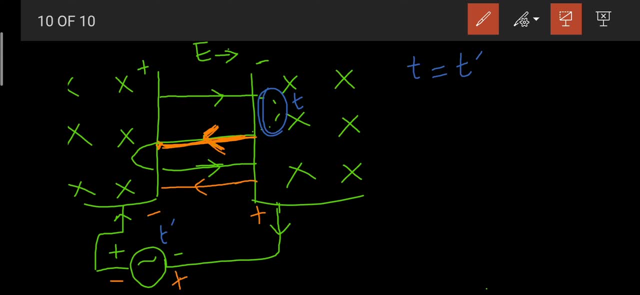 this: how we can determine the value of this t. how can we determine the value of this t? we will definitely do a simple calculation, which we have already done. we already knew all these equations which i have written over here. we already know that v is equal to qrb, as we have calculated earlier in the previous lecture, and omega the value of omega. 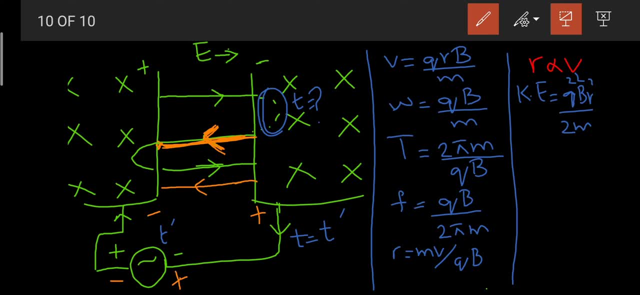 to b cube b by m, the value of t, the value of f, the value of r and the value of kinetic energy as well. and we know this thing: that v and r are directly proportional. so other things like omega t and frequency they are not depending upon the radius kinetic energy is. 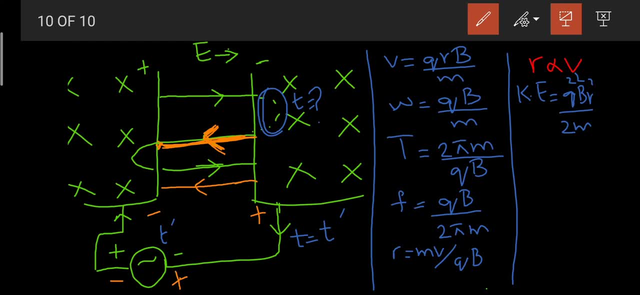 also depending upon velocity, or you can say the radius right. so this time period which we have taken is equal to the time period which we have calculated earlier in the previous lecture. so this is basically the t right, the t which i was talking about, this t. so this is the value. 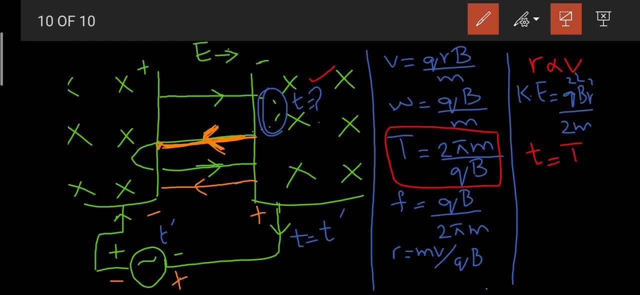 of t, that is 2 pi m divided by q, b. from here we can calculate the value of time period right, how much time required by this charge particle to having a curved path. so this time period would be equal to: obviously m is known because of the charge particle is known charge of that magnitude. 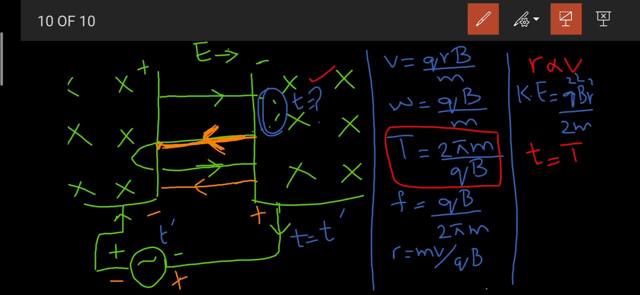 of charge of that particle is known, b supplied is also known. so we can easily calculate the time period. suppose the value of this time period comes out to be. suppose it is 20 millisecond, right, suppose this is 20 millisecond. so if this is 20 millisecond, i will set my oscillator time. 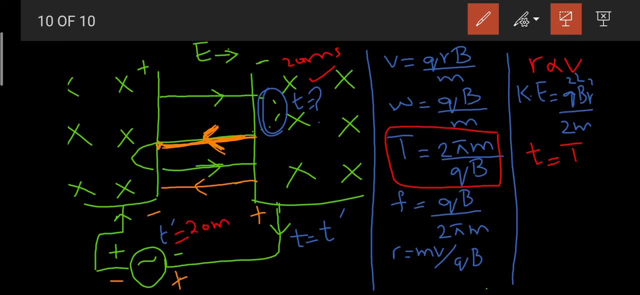 to be 20 millisecond. what is going to happen during that duration, during the 20 milliseconds, what is going to happen? that all the charge particle is will start movement from here to this point and meanwhile, when it starts moving from this point to this point, so starting from here to 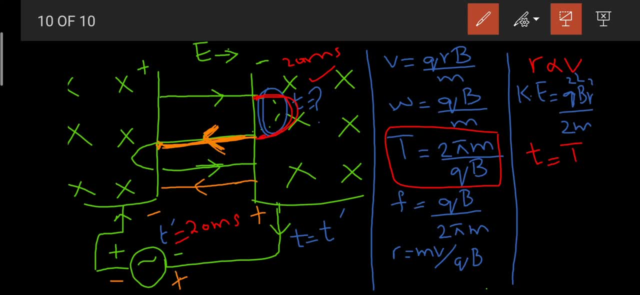 here the time was 20 millisecond. so during that duration, after every 20 milliseconds, what is going to happen? that the oscillator will repeat, or you can say, well, change its polarity. after 20 milliseconds, what is going to happen? that the charged particle will be at this point. 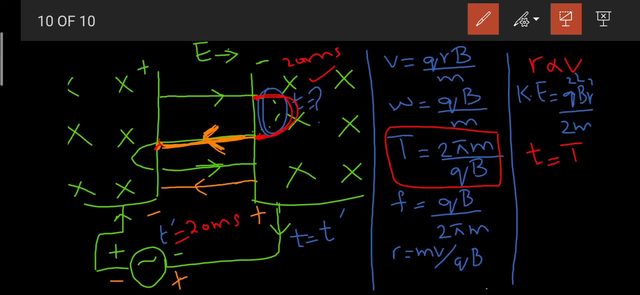 particular point, right, and then again at 20 milli meter, 20 milliseconds. what is going to happen? it will again enter into this particular electric field. then that's how we are going to synchronize e and v with the help of the time period, right? so this is the main thing, and you must be wondering. 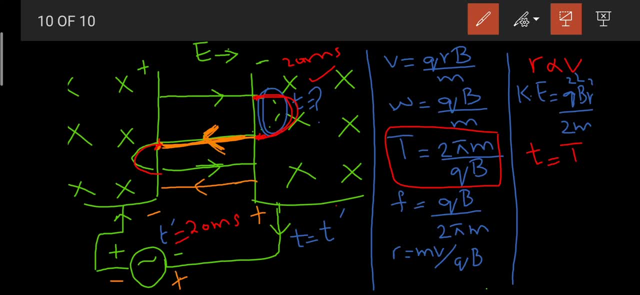 that if you are increasing the velocity and hence the radius is increasing, then definitely the time period should increase. but as you can see in the formula the time period is not depending upon the radius. so for every radius so far, you can say for the whole cyclotron movement of the charged 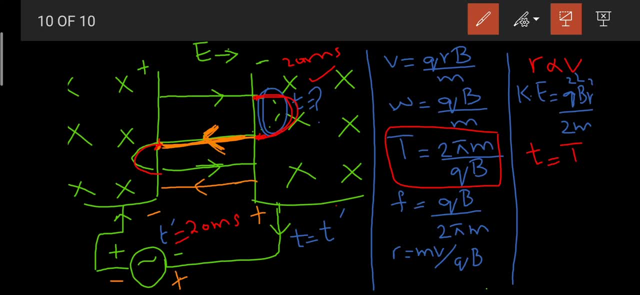 particle time period will remain same. so time period will remain same. so ultimately, what we see, that we are going to get increased velocity at every step when that charged particle is going to enter into the d right. so i hope it is cleared up till now and this kind of synchronization in which e and v are in step, this is known as in step. 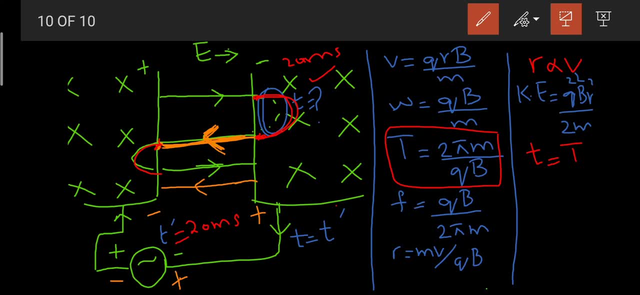 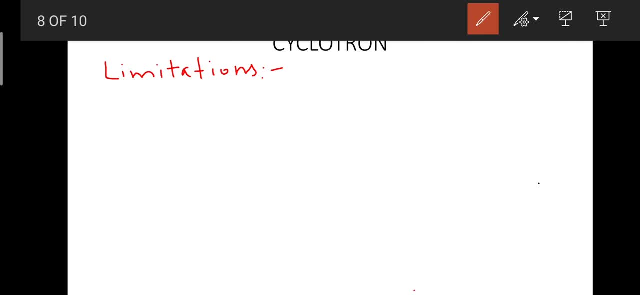 now coming towards the limitations. the now coming towards the limitations. the first limitation of cyclotron is first. limitation of cyclotron is first. limitation of cyclotron is that neutrons for the neutrons, the that neutrons for the neutrons, the that neutrons for the neutrons, the cyclotron is not going to work right. 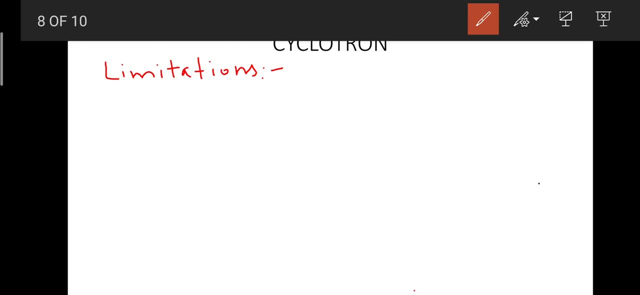 cyclotron is not going to work right. cyclotron is not going to work right why? because cyclotron only accelerates to. why? because cyclotron only accelerates to. why? because cyclotron only accelerates to charge particles. right if the there is no charge particles. right if the there is no. 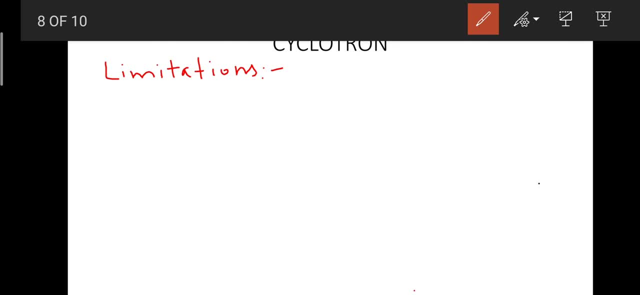 charge particles, right. if the there is no charge, it will. it won't definitely charge it will. it won't definitely charge it will. it won't definitely accelerate in the electric field. so the accelerate in the electric field, so the accelerate in the electric field. so the first limitation is that if Q equals to 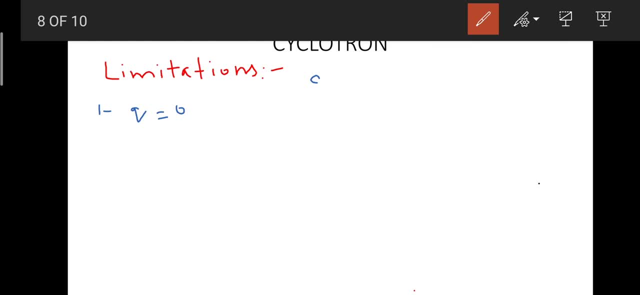 first limitation is that if Q equals to. first limitation is that if Q equals to 0, then definitely. if you would be equal 0, then definitely. if you would be equal 0, then definitely. if you would be equal to 0, right, and if B is also be equal to. 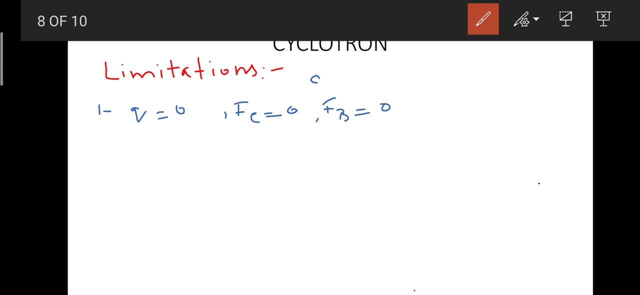 to 0 right, and if B is also be equal to to 0, right, and if B is also be equal to 0, so it is not going to work for the 0, so it is not going to work for the 0, so it is not going to work for the neutral particles right. number two is: 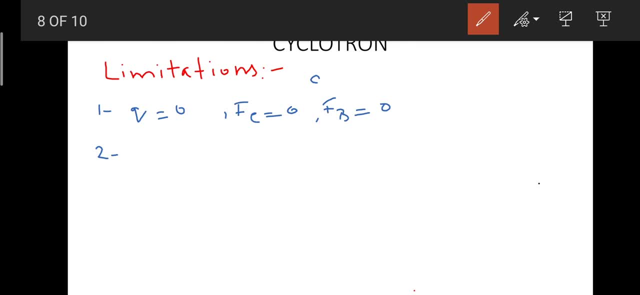 neutral particles. right number two is neutral particles. right number two is that I have become to know and the that I have become to know and the that I have become to know. and the question, that question, that question that: how much velocity can we increase like a? how much velocity can we increase like a? 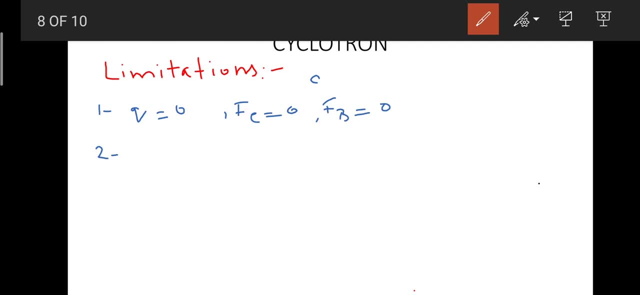 how much velocity can we increase? like a velocity is increasing continuously, like velocity is increasing continuously. like velocity is increasing continuously, like from V to 2 V, then 2 V to 3 V and up to. from V to 2 V, then 2 V to 3 V and up to. 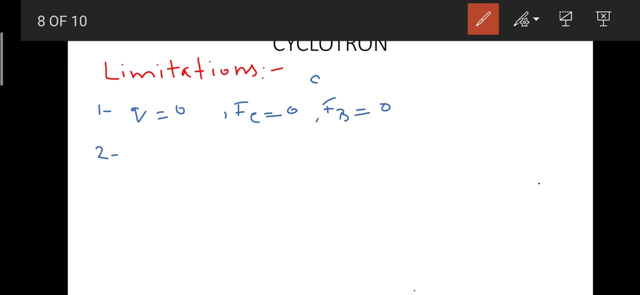 from V to 2 V, then 2 V to 3 V and up to a thousand value it can go. what is the a thousand value it can go? what is the a thousand value it can go? what is the last limit to which we can increase the? 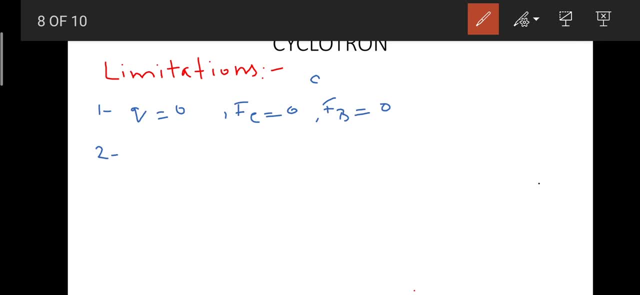 last limit to which we can increase, the last limit to which we can increase the velocity. can it be equal to the speed of velocity? can it be equal to the speed of velocity? can it be equal to the speed of light it is? is it possible? no, it's not. 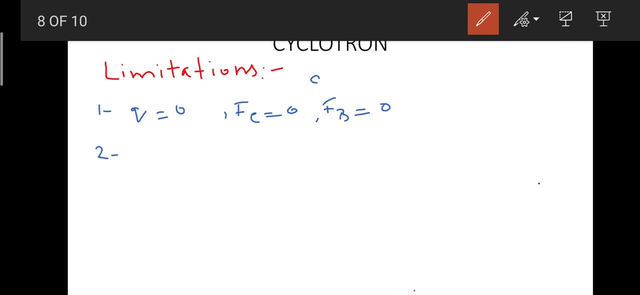 light it is. is it possible? no, it's not. light it is. is it possible? no, it's not possible. right why it is not possible. possible. right why it is not possible. possible. right why it is not possible. because we have put our effort in. because we have put our effort in. 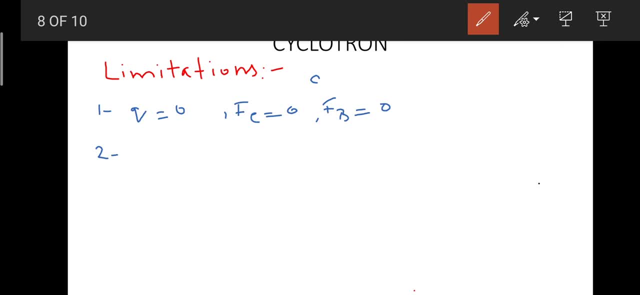 because we have put our effort in putting E and V to be synchronized, to be putting E and V to be synchronized, to be putting E and V to be synchronized, to be remain in step, but as the velocity is remain in step. but as the velocity is remain in step, but as the velocity is getting higher, that consider that. 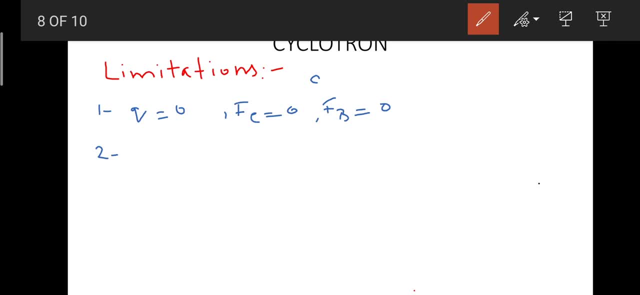 getting higher, that consider that getting higher, that consider that velocity has become 90% of the speed of velocity, has become 90% of the speed of velocity, has become 90% of the speed of light, or 80% of the speed of light. what? 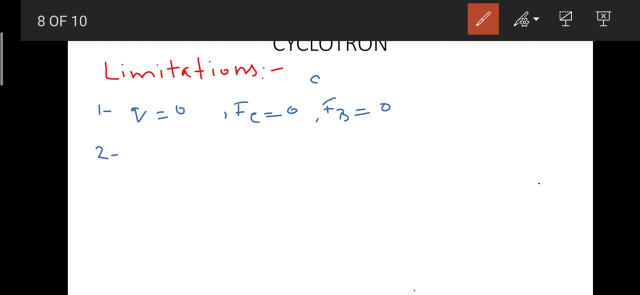 light or 80% of the speed of light? what light or 80% of the speed of light, what is going to happen? that at higher? is going to happen that at higher? is going to happen that at higher velocity, when V increases, like if V is? 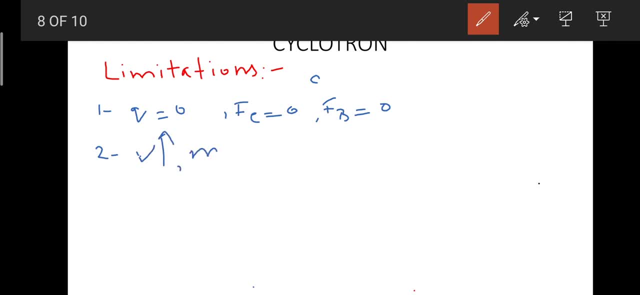 velocity when V increases, like if V is velocity when V increases, like if V is in, is going to be increased. the in is going to be increased. the in is going to be increased. the relativistic mass is going to be. relativistic mass is going to be. 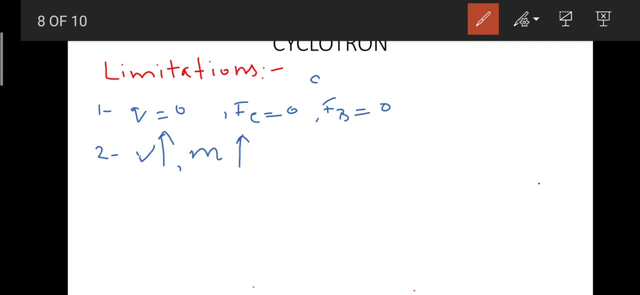 relativistic mass is going to be increased right and when the increased right and when the increased right and when the relativistic mass increases time period. relativistic mass increases time period. relativistic mass increases time period also increases right. these relativistic also increases right. these relativistic. 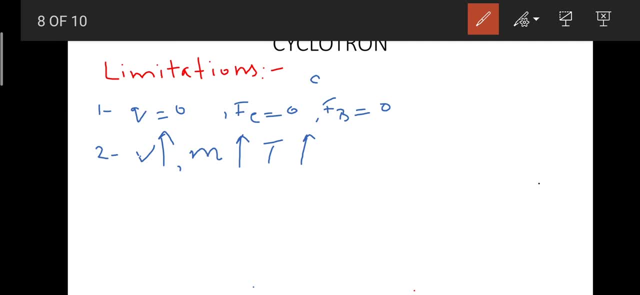 also increases. right, these relativistic effects, you will definitely going to effects. you will definitely going to effects, you will definitely going to learn in chapters ahead. okay so, because learn in chapters ahead. okay so, because learn in chapters ahead. okay so, because of the relativistic effect, of the relativistic effect, 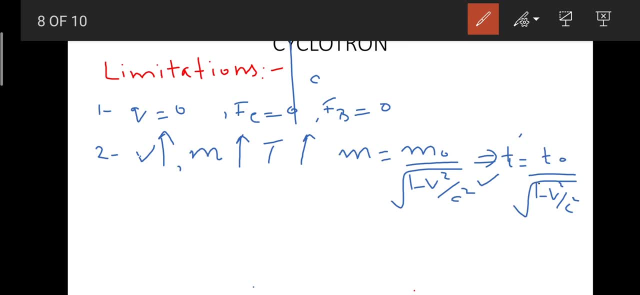 of the relativistic effect. what is going to happen that, if we are? what is going to happen that if we are? what is going to happen that if we are increasing the value of V, like, suppose increasing the value of V, like, suppose increasing the value of V, like, suppose we are moving it to 90% of the speed of we are moving it to 90% of the speed of. we are moving it to 90% of the speed of light, or 70% of the speed of light, or 80% light, or 70% of the speed of light, or 80%. 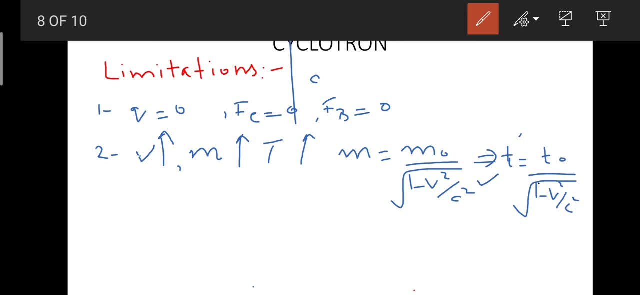 light, or 70% of the speed of light, or 80% of the speed of light. so if I'm of the speed of light, so if I'm of the speed of light, so if I'm increasing the value of V relativistic, increasing the value of V relativistic, 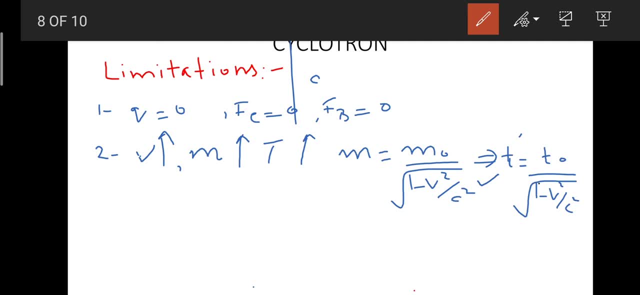 increasing the value of V. relativistic effects will definitely come into action. effects will definitely come into action. effects will definitely come into action. and these relativistic effects you're, and these relativistic effects you're, and these relativistic effects you're going to run. learn in chapter called 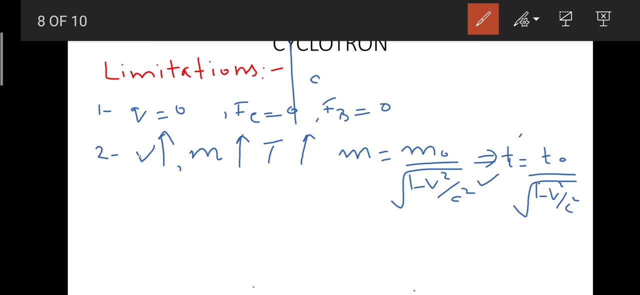 going to run. learn in chapter called going to run. learn in chapter called modern physics. giving you a short chunk modern physics. giving you a short chunk modern physics. giving you a short chunk of review of that. these are the formulas of review of that. these are the formulas. 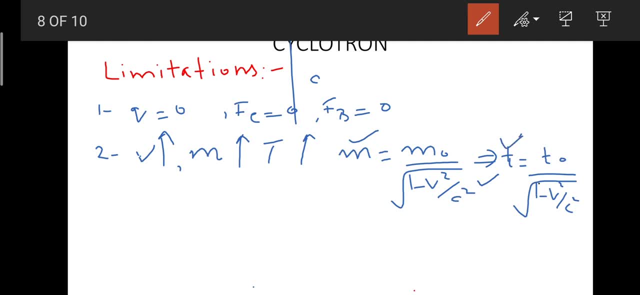 of review of that. these are the formulas for a relativistic mass and relativistic for a relativistic mass and relativistic for a relativistic mass and relativistic time. so you can see in this formulas time, so you can see in this formulas time. so you can see in this formulas that if you are going to increase the 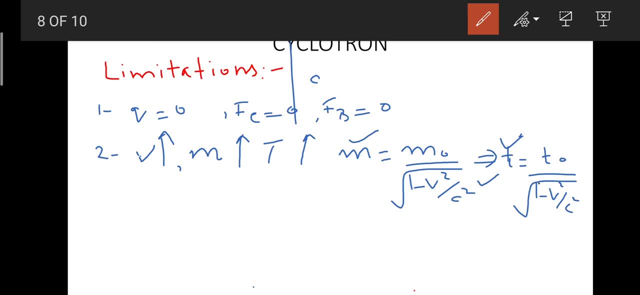 that, if you are going to increase the, that, if you are going to increase the value of V, what is going to happen? value of V: what is going to happen? value of V: what is going to happen overall, the value of this mass would. overall, the value of this mass would. 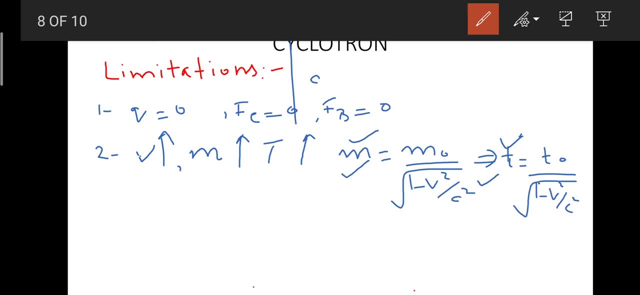 overall, the value of this mass would increase, right? this relativistic mass is increase, right? this relativistic mass is increase, right? this relativistic mass is going to be increased. and if you going to be increased, and if you going to be increased, and if you increase the value of these, V square over. 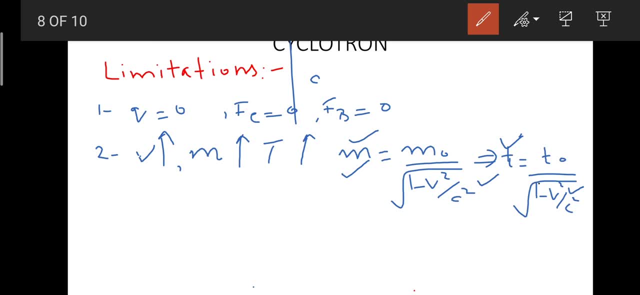 increase the value of these V square over. increase the value of these V square over, here taking the square and then here taking the square, and then here taking the square, and then increasing that value, then 1 minus that. increasing that value, then 1 minus that. increasing that value, then 1 minus that. increased answer and taking the under. increased answer and taking the under increased answer and taking the under root. this will reduce the value and root. this will reduce the value and root. this will reduce the value. and what you met you: what is going to happen. what you met you: what is going to happen. 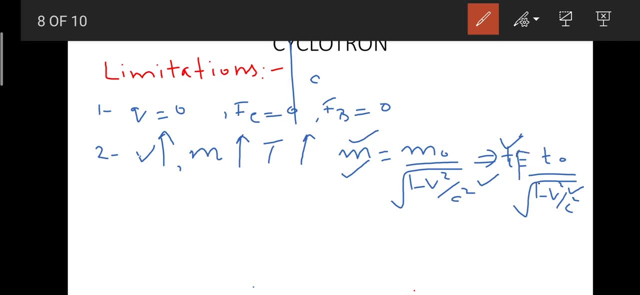 what you met you. what is going to happen? this T would also increase. so if T is this, T would also increase. so if T is this, T would also increase. so if T is going to be increased, which we earlier going to be increased, which we earlier going to be increased, which we earlier had mentioned, that this time period, 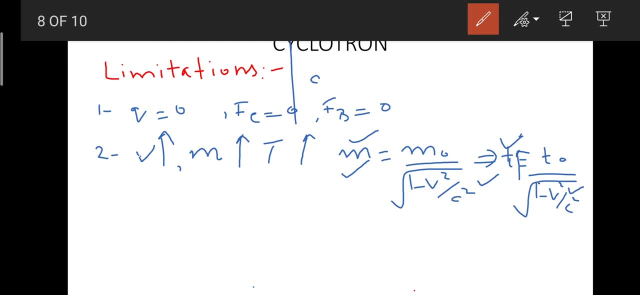 had mentioned that this time period had mentioned that this time period remains constant throughout. the remains constant throughout. the remains constant throughout the cyclotron movement. now the T will cyclotron movement, now the T will cyclotron movement. now the T will definitely increase at higher speed now. 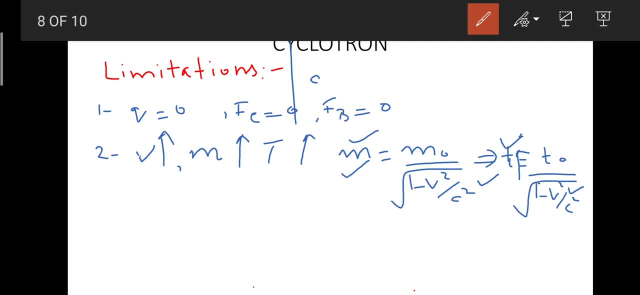 definitely increase at higher speed now. definitely increase at higher speed now at higher speeds. the if T is increased at higher speeds. the if T is increased at higher speeds. the if T is increased e and we won't be longer in step they. e and we won't be longer in step they. 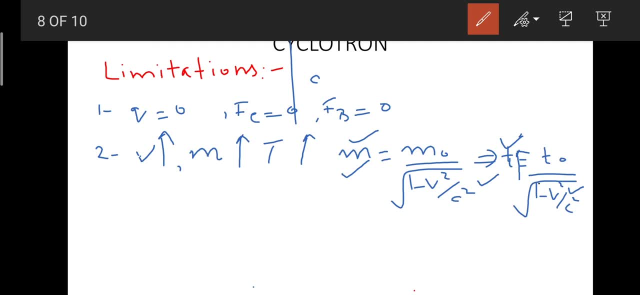 e and we won't be longer in step. they will get out of step and that's how the will get out of step and that's how the will get out of step and that's how the velocity restarts and no further. velocity restarts and no further. 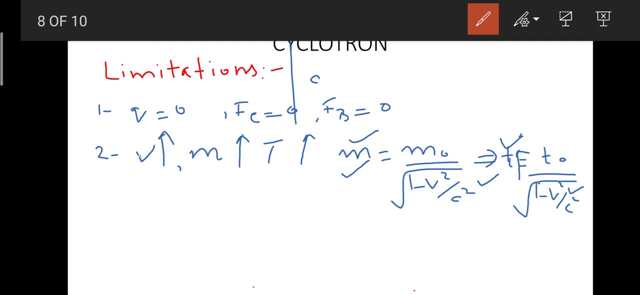 velocity restarts and no further acceleration would occur. so we can, acceleration would occur. so we can. acceleration would occur so we can receive the velocity to a fixed value. receive the velocity to a fixed value, receive the velocity to a fixed value and after that value there will be no. 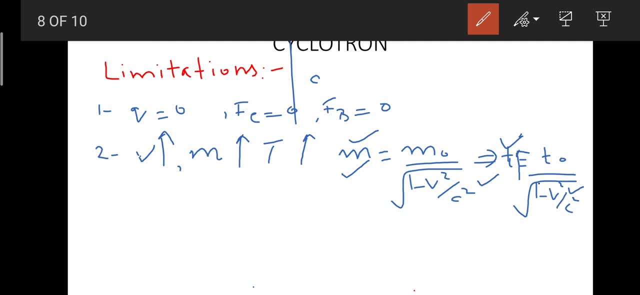 and after that value there will be no, and after that value there will be no further acceleration. right now. the third further acceleration. right now. the third further acceleration. right now. the third limitation. third limitation is that it limitation. third limitation is that it limitation. third limitation is that it is not applicable on electrons right, not? 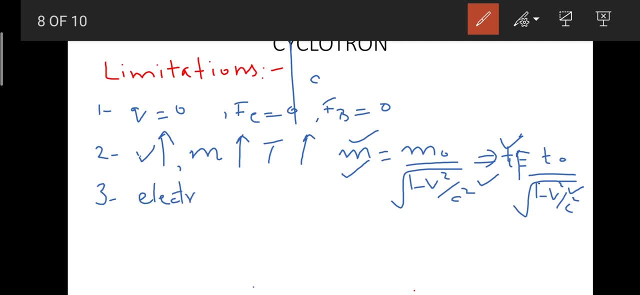 is not applicable on electrons right not is not applicable on electrons right. not applicable on electrons. so we cannot applicable on electrons right. not applicable on electrons right. not introduce electrons in cyclotron. why introduce electrons in cyclotron? why introduce electrons in cyclotron? why, because the mass of electron is very 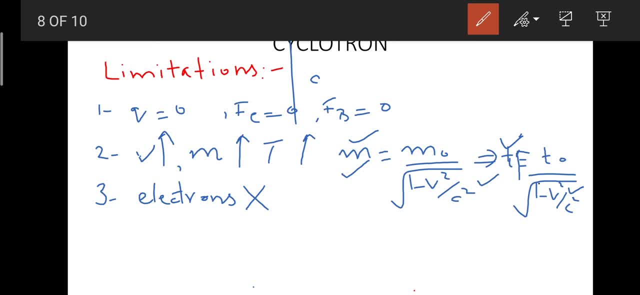 because the mass of electron is very, because the mass of electron is very, very less as compared to the positive, very less as compared to the positive, very less as compared to the positive particle that is considered even particle that is considered even particle that is considered even consider a proton or any like hydrogen. 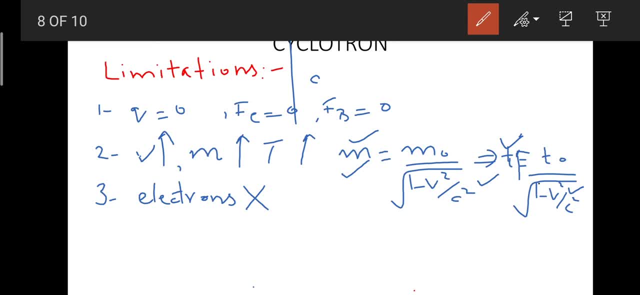 consider a proton or any like hydrogen. consider a proton or any like hydrogen, ion or the helium ion and so on. ion or the helium ion and so on. ion or the helium ion and so on. electrons are going, are having a very. electrons are going, are having a very. 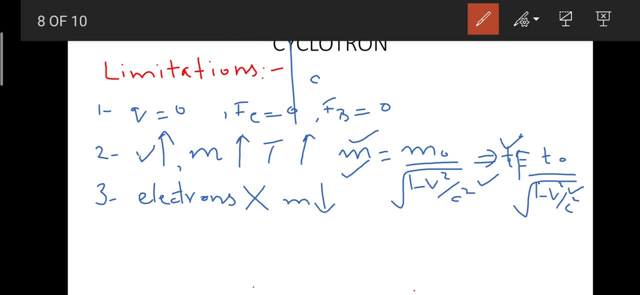 electrons are going are having a very less mass right, very less mass, which is less mass right, very less mass, which is less mass right, very less mass, which is going to be the value of the order of going to be the value of the order of going to be the value of the order of minus 31. so, in this case, what is going to? 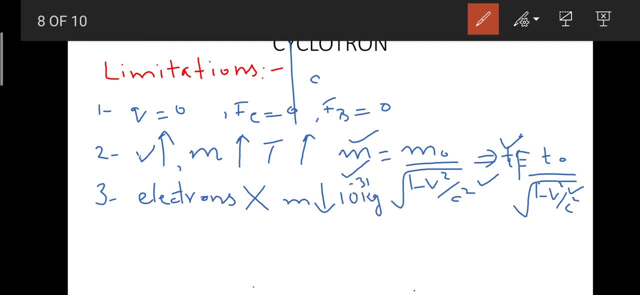 minus 31. so in this case, what is going to minus 31? so in this case, what is going to happen with this? less mass velocity is happen. with this, less mass velocity is happen with this, less mass velocity is going to be increased so much, right? so? 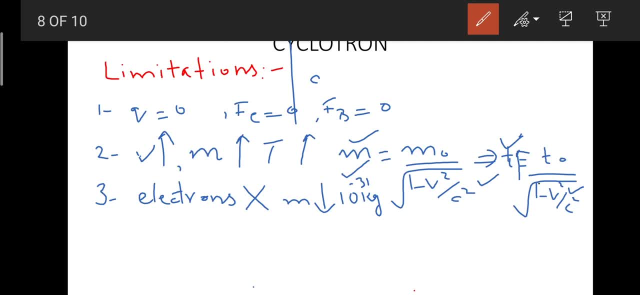 going to be increased so much, right so. going to be increased so much, right so. these higher velocities are unable to be. these higher velocities are unable to be. these higher velocities are unable to be taken in like. we cannot record those taken in like we cannot record those. 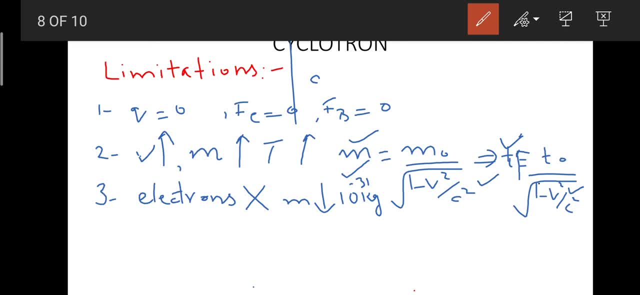 taken in like. we cannot record those values, we cannot achieve those values, values. we cannot achieve those values, values. we cannot achieve those values because it gets a higher high, because it gets a higher high, because it gets a higher high. achieving a higher velocity value in a. achieving a higher velocity value in a. 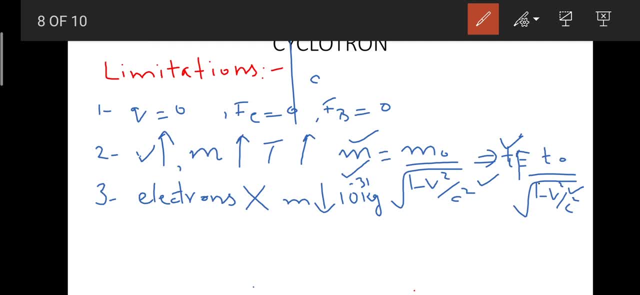 achieving a higher velocity value in a very small interval of time. and nothing, very small interval of time, and nothing, very small interval of time, and nothing is going to be happen. so we cannot, is going to be happen. so we cannot, is going to be happen. so we cannot introduce these electrons in the 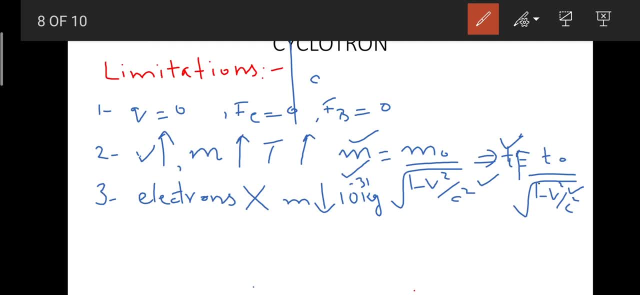 introduce these electrons in the. introduce these electrons in the cyclotron. right next thing that these, the cyclotron. right next thing that these, the cyclotron. right next thing that these the fourth limitation and the last one is fourth limitation and the last one is fourth limitation and the last one is that the higher the positively charged. 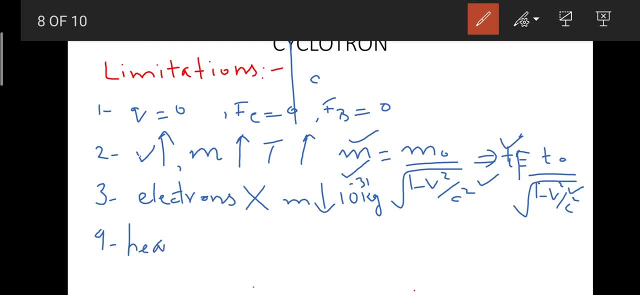 that the higher the positively charged that the higher the positively charged particles with larger mass right. so we particles with larger mass right. so we particles with larger mass right. so we can write that the heavier can write that the heavier can write that the heavier positively charged atoms, like their ions. 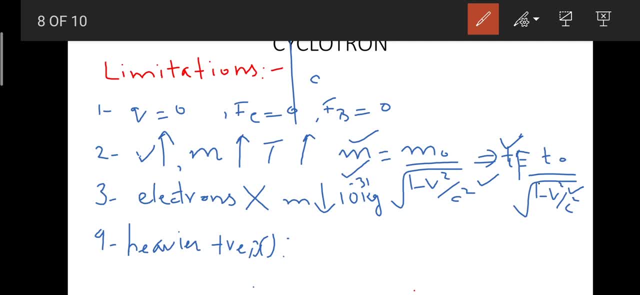 positively charged atoms like their ions. positively charged atoms like their ions- definitely these are also cannot be introduced in. these are also cannot be introduced in. these are also cannot be introduced in cyclotron reason. reason behind is they cyclotron reason. reason behind is they cyclotron reason. reason behind is they are having a large mass and when the 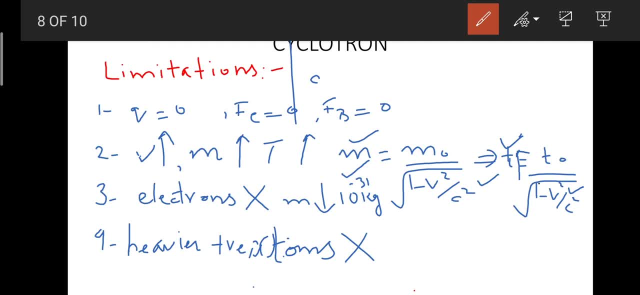 are having a large mass and when the are having a large mass, and when the mass is large, velocity would definitely. mass is large. velocity would definitely mass is large. velocity would definitely increase, but when velocity as a reach to increase. but when velocity as a reach to increase, but when velocity as a reach to near to the. 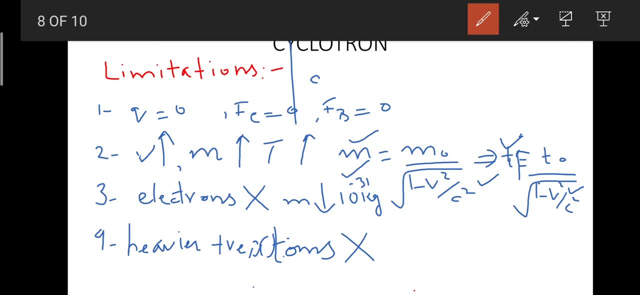 near to the near to the comparable to the speed of light. what is comparable to the speed of light? what is comparable to the speed of light? what is going to happen? time period will going to happen. time period will going to happen. time period will increase when time period will increase. 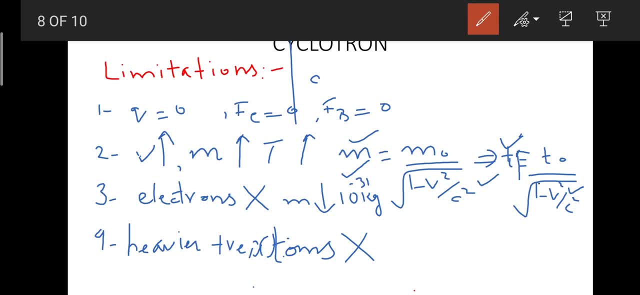 increase when time period will increase, increase when time period will increase. ultimately, what is going to happen? that, ultimately, what is going to happen? that, ultimately, what is going to happen? that E and V will no longer be in synchronized. E and V will no longer be in synchronized. 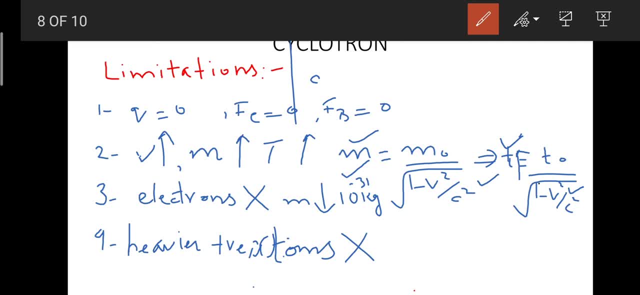 E and V will no longer be in synchronized. they will get out of step and they will get out of step and they will get out of step and ultimately the velocity gets reduced. so ultimately, the velocity gets reduced. so ultimately, the velocity gets reduced. so for the heavier positive atoms, we cannot. 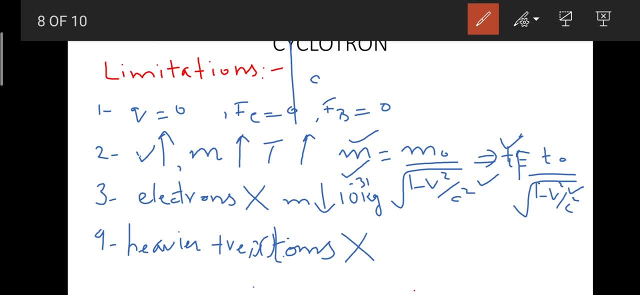 for the heavier positive atoms, we cannot for the heavier positive atoms. we cannot use the cyclotron effect right, so use the cyclotron effect right, so use the cyclotron effect right. so because of these limitations, cyclotrons, because of these limitations, cyclotrons, because of these limitations, cyclotrons are in less usage as a particle. 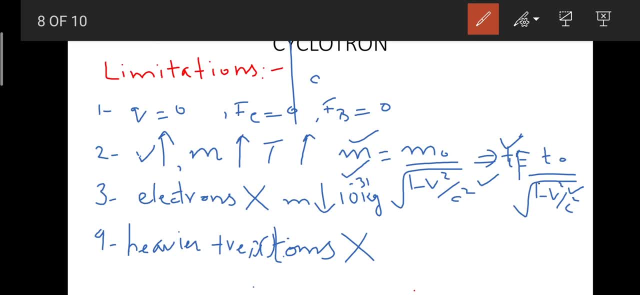 are in less usage as a particle, are in less usage as a particle accelerator. we use to accelerate the accelerator. we use to accelerate the accelerator. we use to accelerate the particles. we use other devices or other particles. we use other devices or other particles. we use other devices or other machines which can provide us the 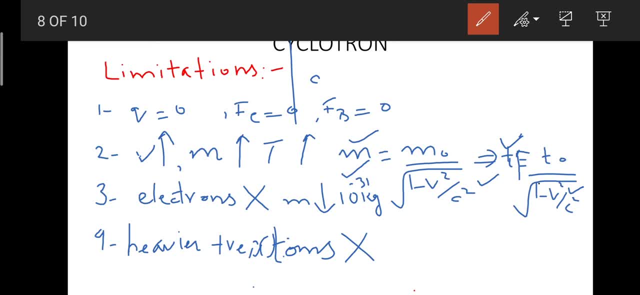 machines which can provide us the machines which can provide us the accelerator for the heavier accelerator, for the heavier accelerator for the heavier positively charged atoms and for the positively charged atoms and for the positively charged atoms and for the electrons as well, coming towards the electrons as well coming towards the. 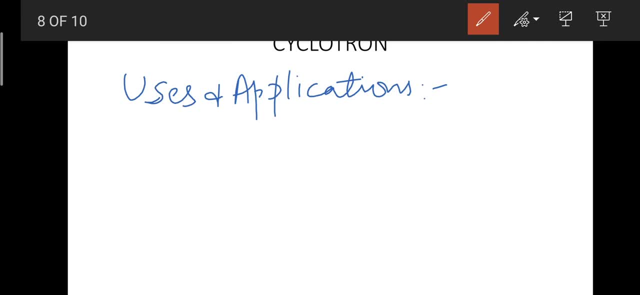 electrons as well, coming towards the users and application users and application users and application. okay, so, what is the first use this? okay, so, what is the first use this? okay, so, what is the first use? this basically can be used as definitely as a. basically can be used as definitely as a. 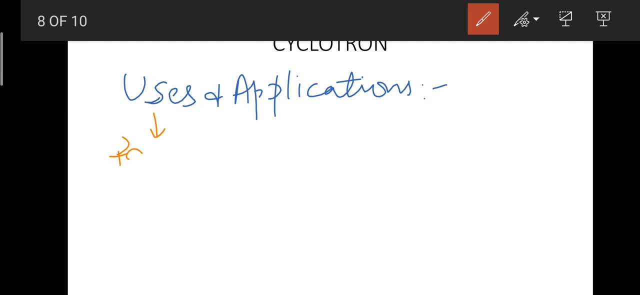 basically, can be used as definitely as a particle accelerator right. so we can use particle accelerator right. so we can use particle accelerator right. so we can use it to accelerate the particles which are it to accelerate the particles which are it to accelerate the particles which are light in way, light and mass having a 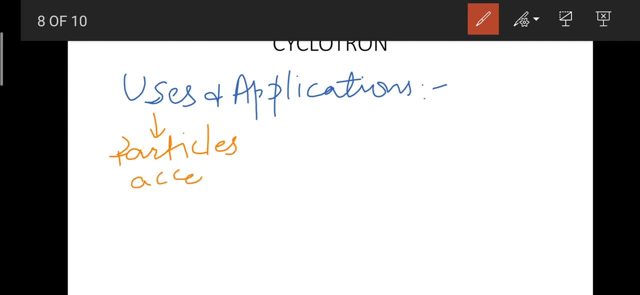 light in way light and mass. having a light in way light and mass. having a smaller mass, so particle it. is it used as smaller mass, so particle it. is it used as smaller mass, so particle it. is it used as a particle accelerator? it is used in a particle accelerator. it is used in. 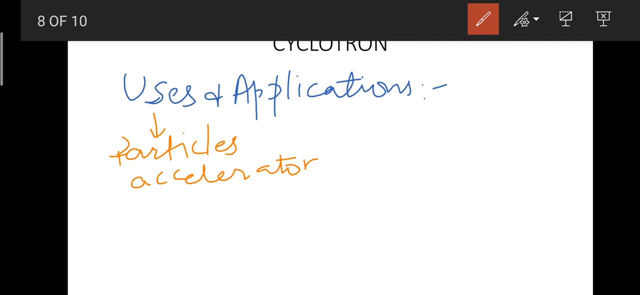 a particle accelerator. it is used in many experiments which are performed in many experiments which are performed in many experiments which are performed in nuclear physics and particle physics, as nuclear physics and particle physics as nuclear physics and particle physics as well. and what are the practical? well, and what are the practical? 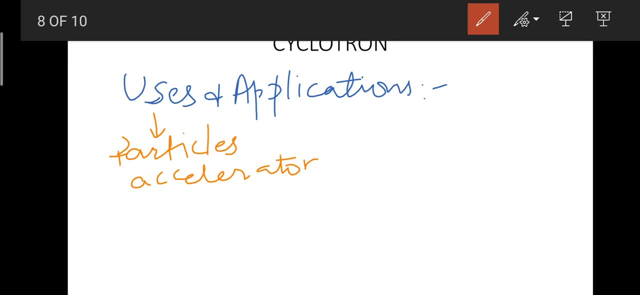 well, and what are the practical applications? one of the application is applications. one of the application is applications. one of the application is the particle accelerator and other. the particle accelerator and other. the particle accelerator and other. application which we observe in medical application, which we observe in medical. 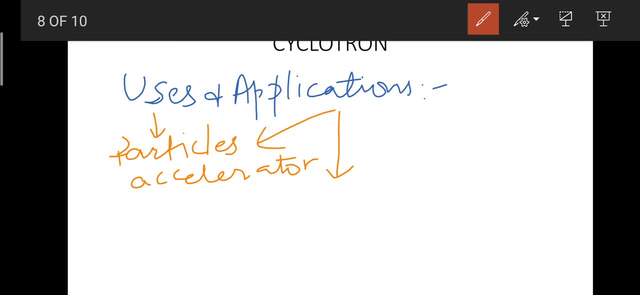 application which we observe in medical field is basically that particle therapy field is basically that particle therapy field is basically that particle therapy is used to treat the cancer and there is is used to treat the cancer and there is is used to treat the cancer and there is also another technique. we are having the 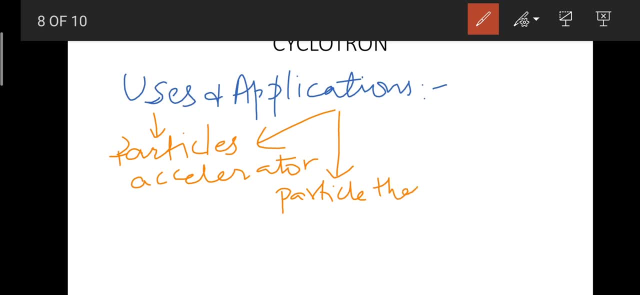 also another technique. we are having the also another technique. we are having the particle therapy to treat cancer and a particle therapy to treat cancer, and a particle therapy to treat cancer and a proton therapy. proton therapy, in which these particle cyclotrons are used right proton, in which these particle cyclotrons are used right proton. 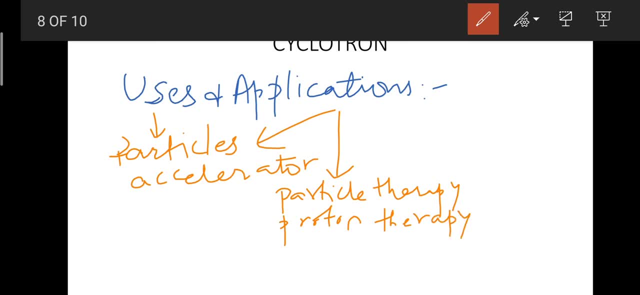 in which these particle cyclotrons are used right proton therapy as well. both of these are used to therapy as well. both of these are used to therapy as well. both of these are used to diagnose the cancer cells. right any diagnose the cancer cells. right any diagnose the cancer cells. right any blockage in the system, like in the. 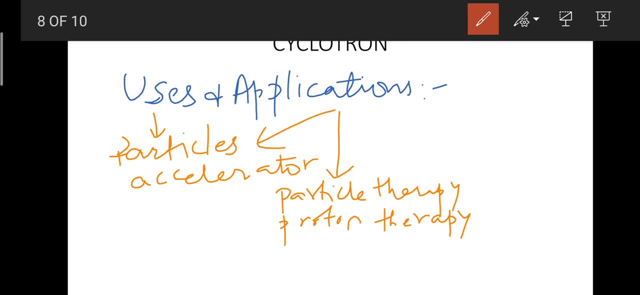 blockage in the system, like in the blockage in the system, like in the circulatory system, and to treat the circulatory system and to treat the circulatory system and to treat the cancer as well, like to treat the cancer, cancer as well, like to treat the cancer. 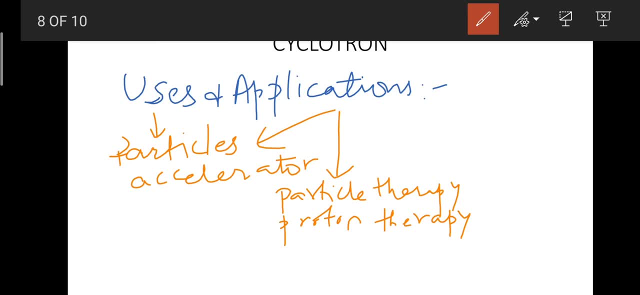 cancer as well. like to treat the cancer means definitely to destroy the cancer, means definitely to destroy the cancer, means definitely to destroy the cancer cells, and again in many of the cells, and again in many of the cells, and again in many of the experiments that are performed in. 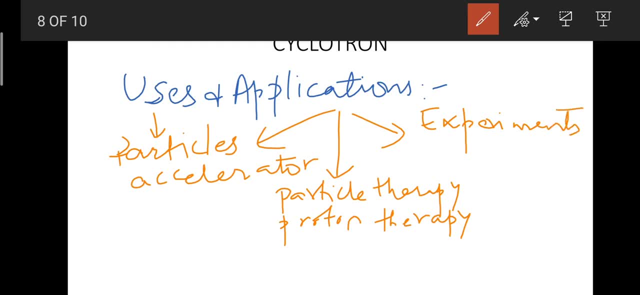 experiments that are performed in, experiments that are performed in nuclear and particle physics: right. so nuclear and particle physics right. so nuclear and particle physics right. so that was the article for today. it is not that was the article for today. it is not that was the article for today. it is not given in your book in so much detail, so 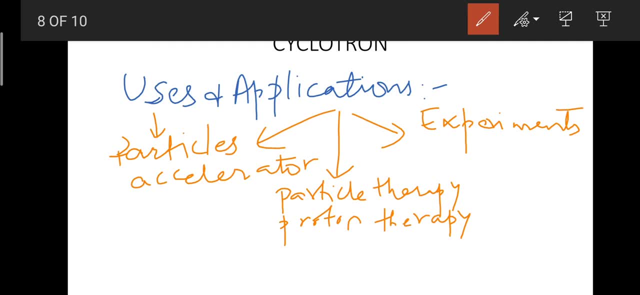 given in your book in so much detail. so given in your book in so much detail, so I've provided in your detail as this is. I've provided in your detail as this is. I've provided in your detail as this is going to help you in your entry test as going to help you in your entry test as going to help you in your entry test as well. thank you so much for today's well. thank you so much for today's well. thank you so much for today's article. Allah Hafiz.